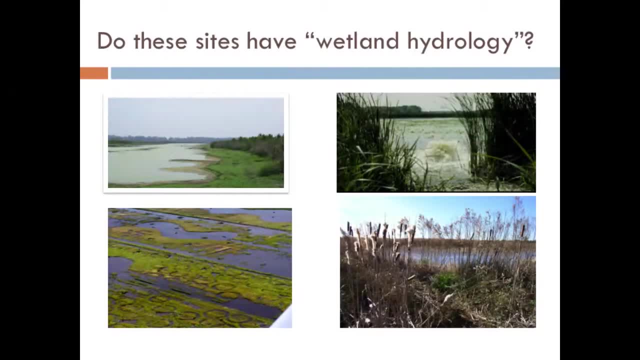 The ultimate success of that project will depend on hydrology being able to support the plant community. Now how do we determine whether hydrology is successfully restored? We've got the tools needed. We've got automated wells. We've got rain gauges. 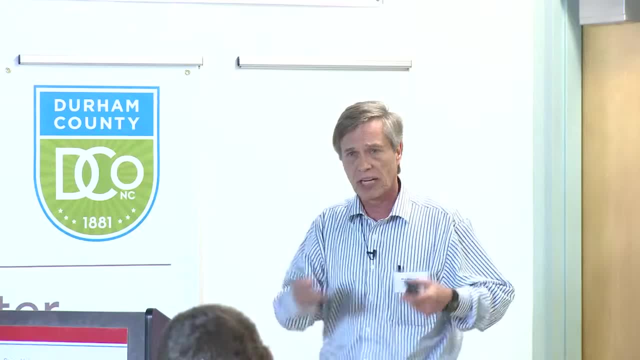 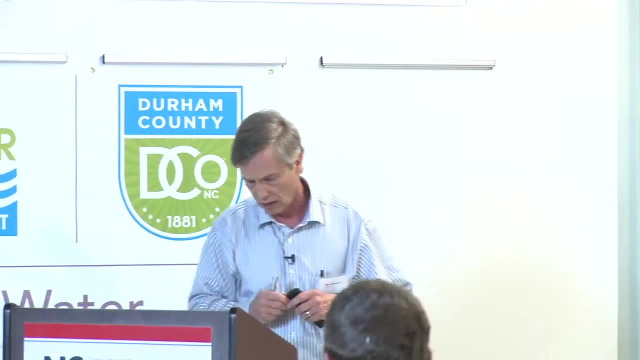 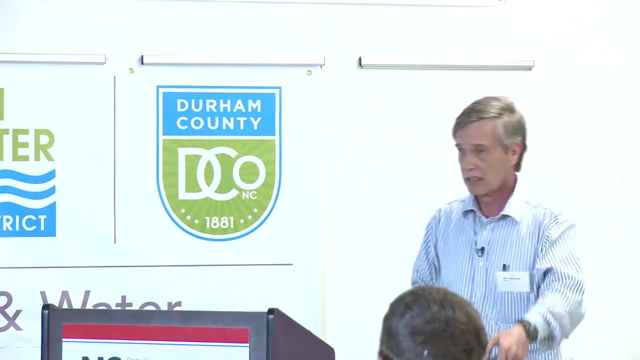 Now, up until Kevin's talk, I thought because we had the tools, we always collected the data. We will collect it, I guess, if our monitoring budget is sufficient. So in general, I think we've got the data. The biggest problem I see is that we do not have any method. 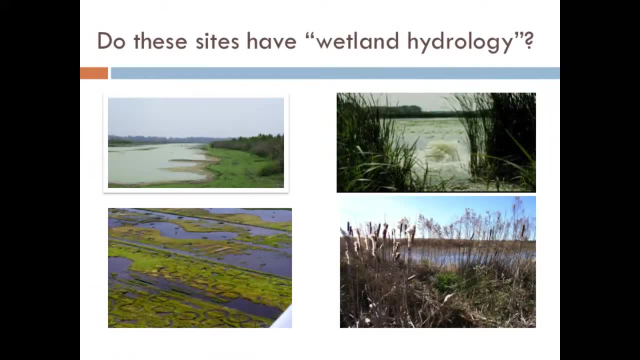 for evaluating that data. So for these restored sites, one created- I'd ask the question: do they meet wetland hydrology? Well, in many cases we have the data on water table fluctuations of rainfall, but we don't have an agreed upon technical standard for interpreting it. 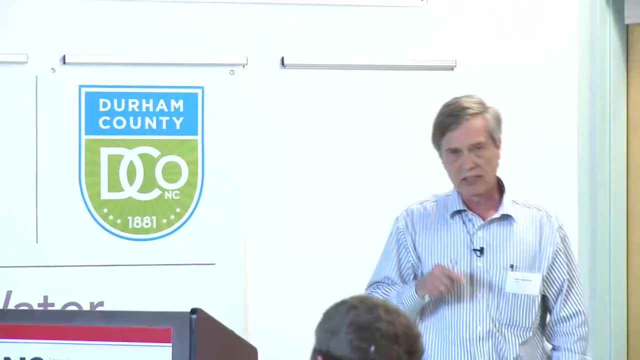 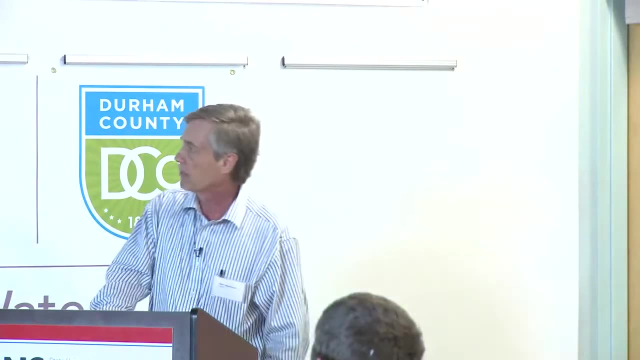 So today I want to discuss a proposed technical standard for identifying appropriate wetland hydrology and restoration sites. Now, as I get into this, let me give you some background. It was developed for the North Carolina River, The North Carolina Ecosystem Enhancement Program. 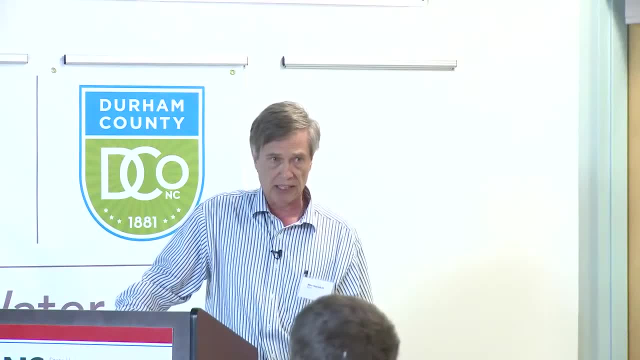 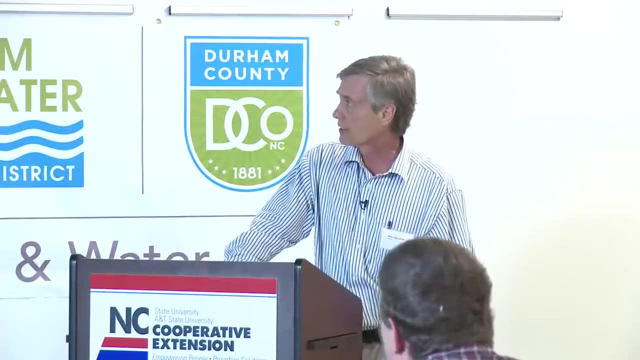 And so it's not an official policy as yet because we've just- it's basically hot off the press and still in discussion. It's a proposal, so it's not going to be implemented immediately And I want you to remember that I'm an academic. 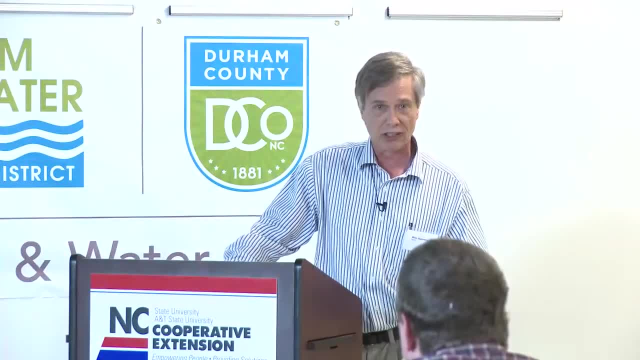 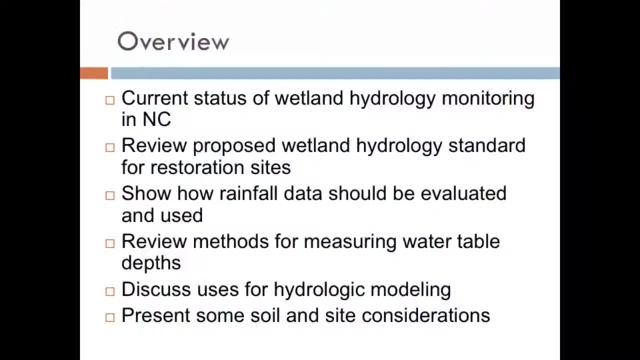 I do not have the power to implement it myself. I'm only the messenger in this case. okay, The actual decision on implementation will come from a North Carolina state government agency. Now, in this talk, I'm going to try to do six things for you. 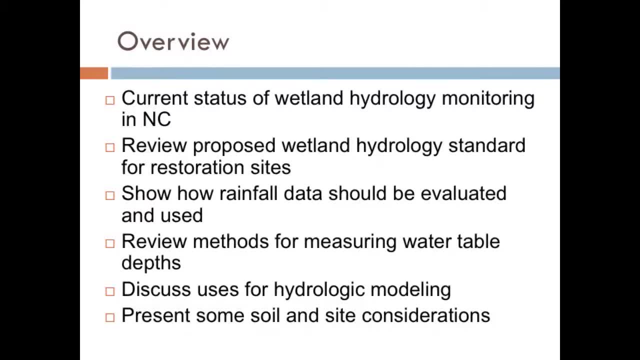 First discuss the status of wetland hydrology monitoring in North Carolina, Then review the proposed hydrology standard that we developed for EEP. I'll show how rainfall should be evaluated. talk about measuring water tables, methods for doing that, a little bit of discussion on hydrologic modeling and how that can be involved with evaluating restoration sites. 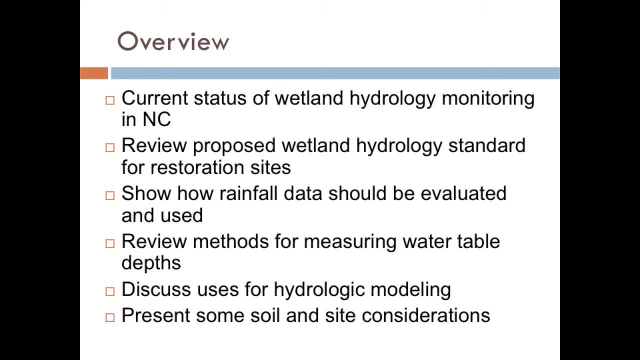 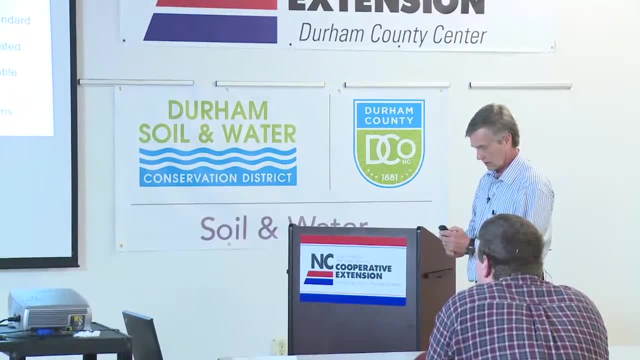 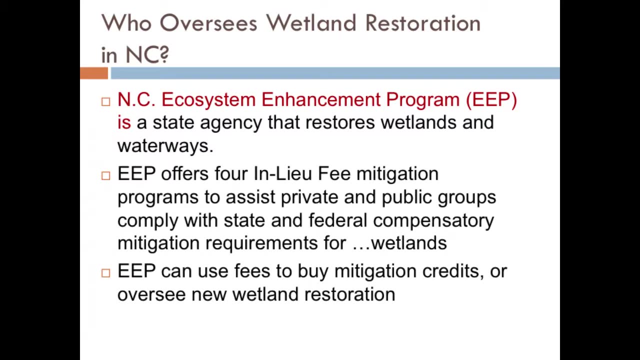 and then present some soil and site considerations, Like before. if you've got questions, just let me know. Okay, there we go. All right now. who oversees wetland restoration in North Carolina? You've heard the term North Carolina Ecosystem Enhancement Program. I think throughout, at least today, I've heard it. 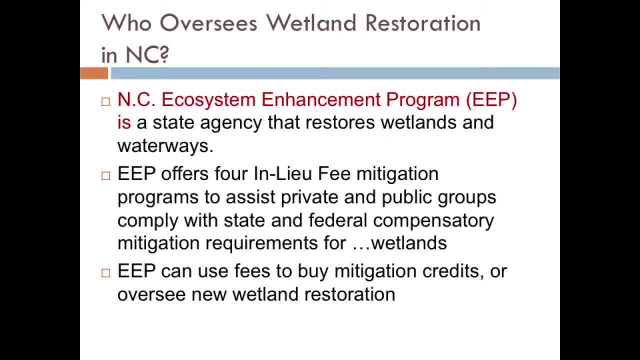 It is a state agency that is responsible for restoring wetlands as well as streams. It offers four in lieu fee mitigation programs to assist both private and public landowners with their compensatory mitigation requirements. In short, EEP will collect money from people that need to restore wetlands. 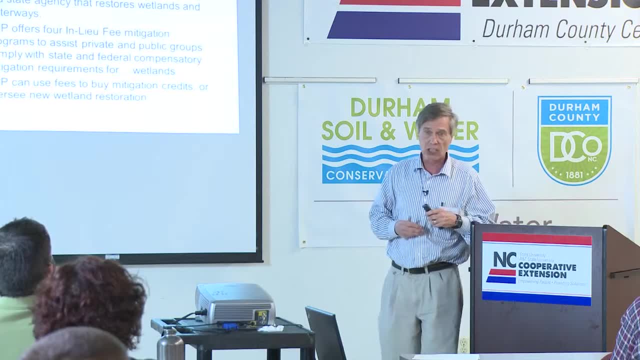 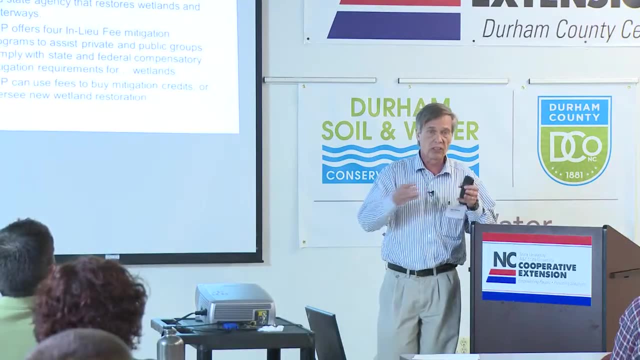 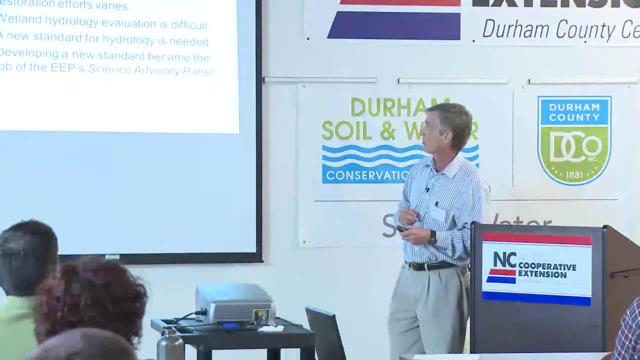 They can take the money and give it, or buy credits from a mitigation bank, and it's pretty much straightforward. On the other hand, they can hire a consulting company- maybe some of you folks- to build a restored wetland. In that latter case, though, they have to evaluate whether the restoration is successful or not. 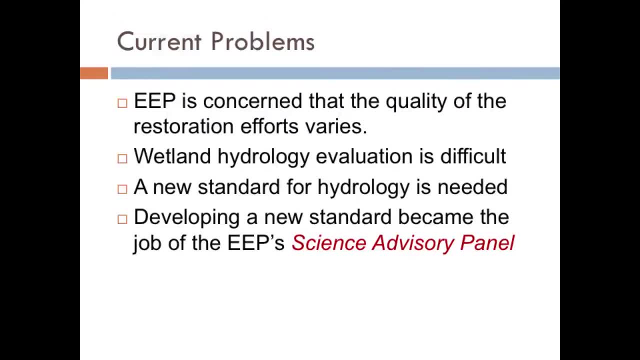 The current problems that EEP has told some of us is that they're concerned about the quality of the restoration. The hydrology is the most difficult thing to evaluate, and they don't have good tools for evaluating it at this time, And so a new standard for hydrology was needed, and that job was given to the EEP's relatively newly appointed science advisory panel. 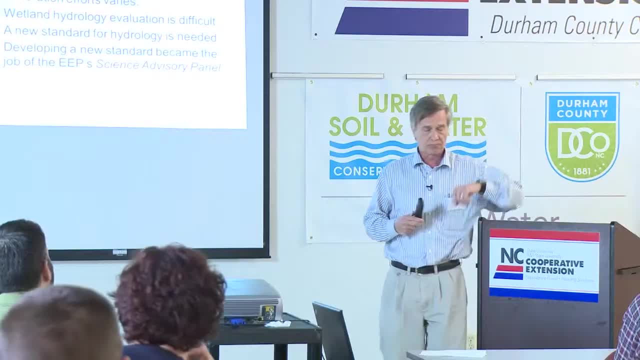 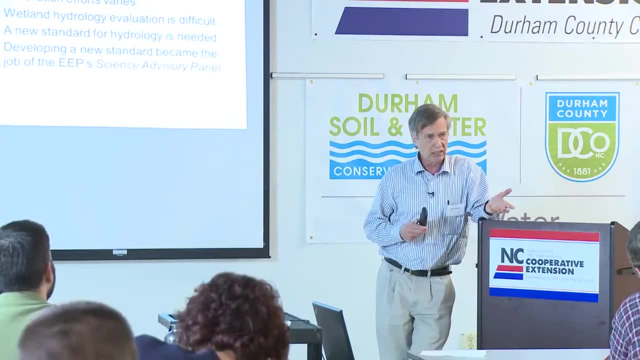 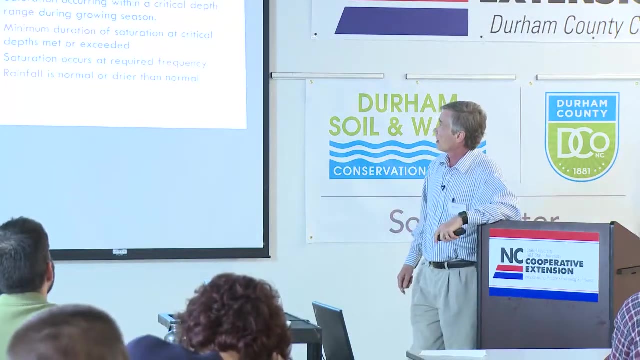 It's a group of academics- I'm on it, Kurt Richardson's on it, Mac Halp, representing EEP, is on it, And a number of others from both the regulatory state, government agency and academia were assigned the job of coming up with a new hydrology standard. 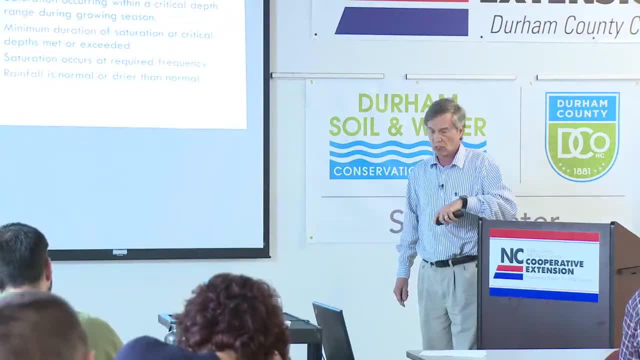 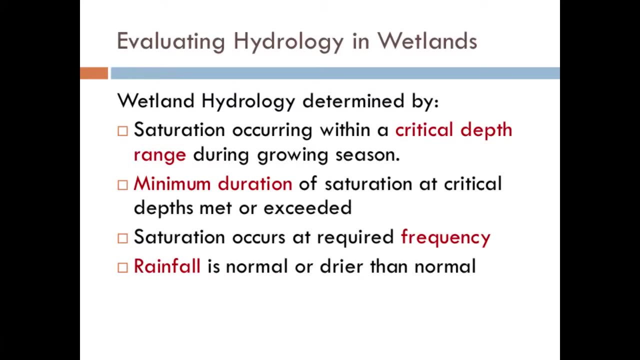 So what do you look for? if you're evaluating hydrology, What do you have to specify? Well, I'm going to be dealing with high water table soils. I'm not going to be dealing with flooding or coastal conditions. In that sense, we need to identify a critical depth where we want saturation to occur. 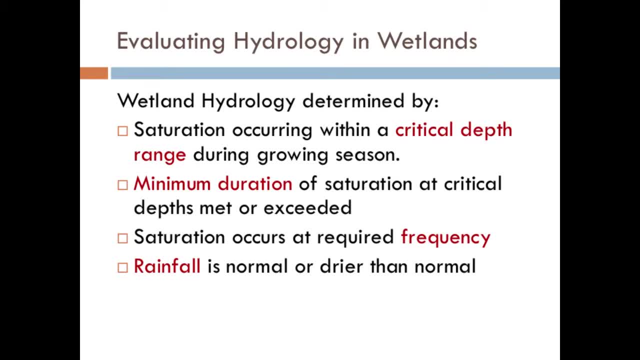 and this usually will occur during the day. It will occur during the growing season. You'll need to specify a minimum duration of saturation, how long you want that critical depth of saturation at the critical depth to be met, as well as how often, how many years out of ten. 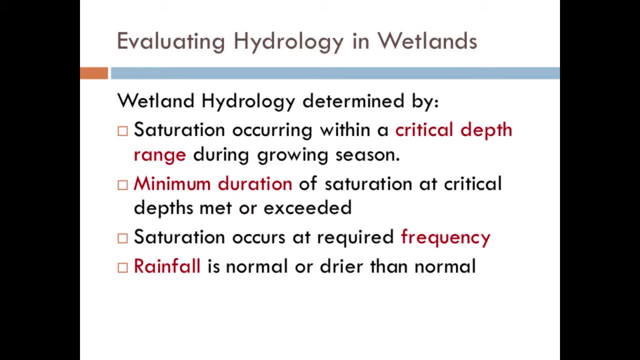 Now, if you have short records of water table levels, you may have to interpret the data by considering the rainfall and look to see if it's normal, drier than normal or whatever, And so these aspects have to be built into your hydrology standard. 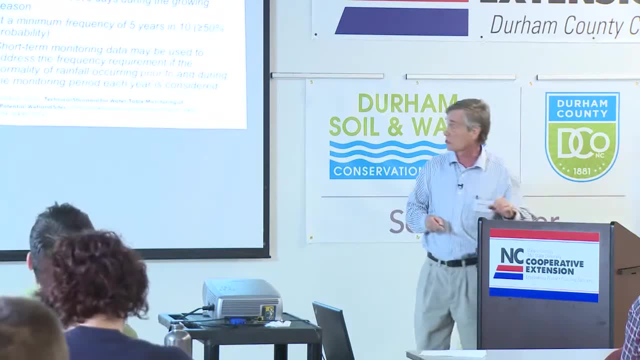 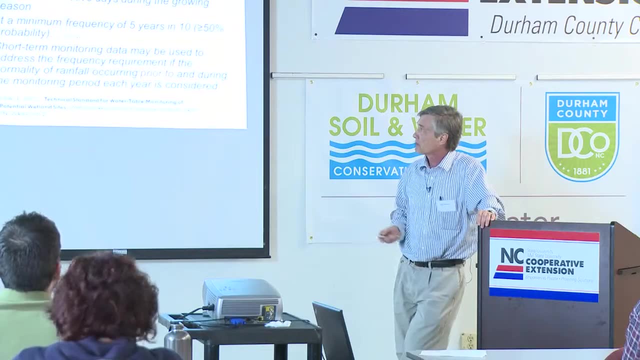 We don't have to start from scratch, or we didn't have to start from scratch on this. The Corps of Engineers has proposed a wetland hydrology technical standard. This came out in 2005, and it's shown here. I should mention that this is for problematic sites. as I understand it, 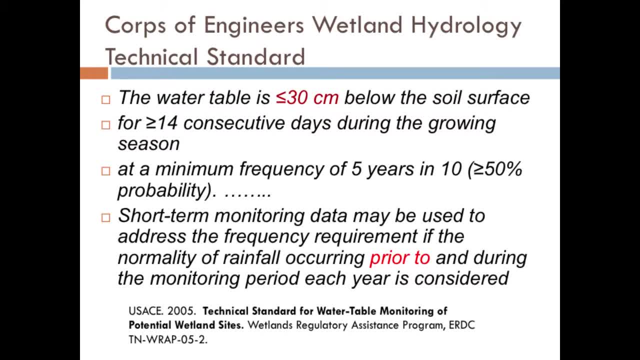 And in my opinion it's well-suited for the wetland edge, Not identifying a wetland in the wettest part or the middle, but looking at the edge. The standard says the water table is within 30 centimeters deep. 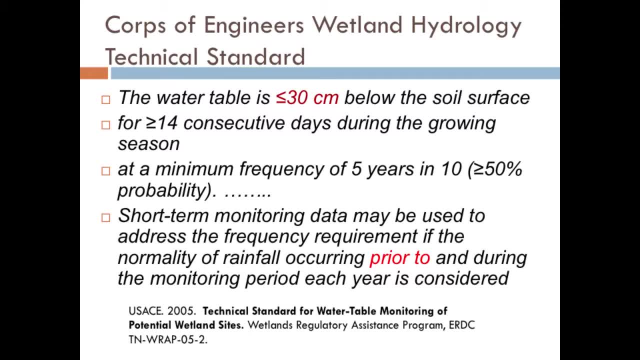 It says the water table is within 30 centimeters of the surface for 14 consecutive days or more during the growing season, at a minimum frequency of five years in ten, or a probability of 50%. I'm going to keep getting back to this latter statement. here the next statement. 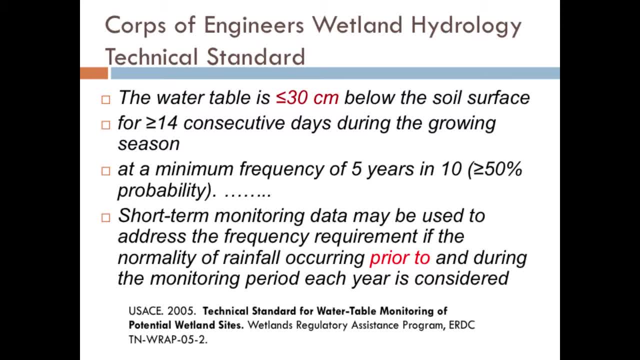 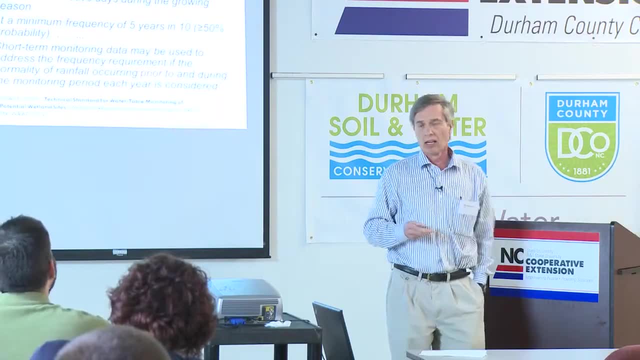 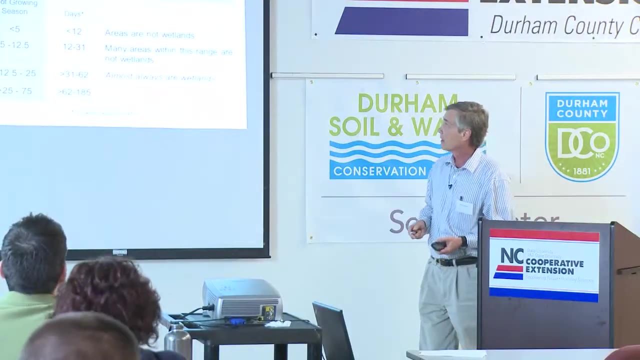 It says short-term monitoring, that is, data collected over a period less than ten years long, can be used to address the frequency if the normality of rainfall occurring prior to and during the monitoring period each year is considered. Need I say more? Well, I'll be talking more about this later, because I think that's probably the most critical part of their entire standard. 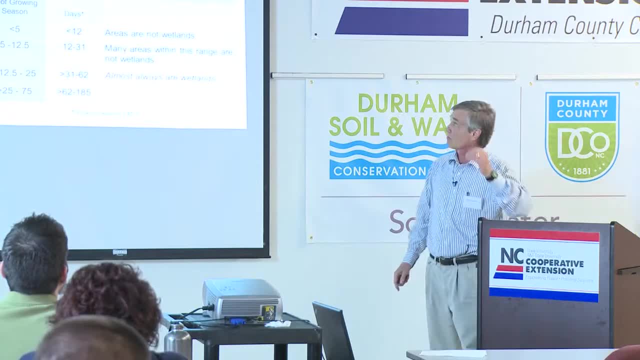 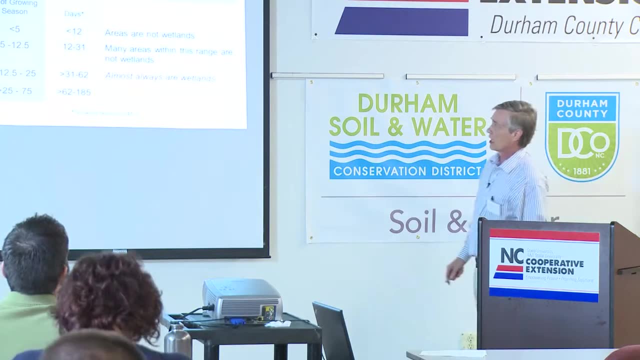 Now I said you have to specify a duration. What are some of the durations that have been used? If you go back to the 87 Wetlands Delineation Manual, they took a stab at showing what durations of hydrology are appropriate for wetlands. 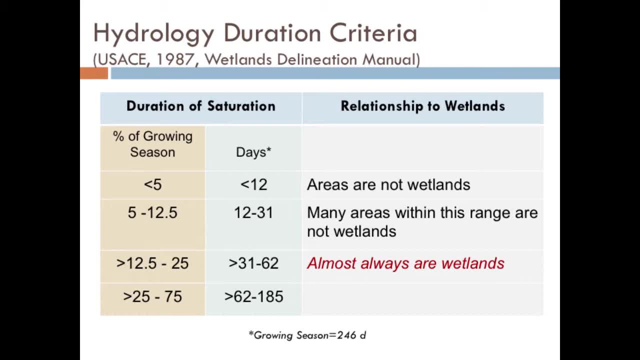 And I've just copied that stuff right here. I've got a growing season here as one measure of duration, of saturation. I've translated that into days, assuming a growing season of about 246 days. and then the comments from the 87 Manual. 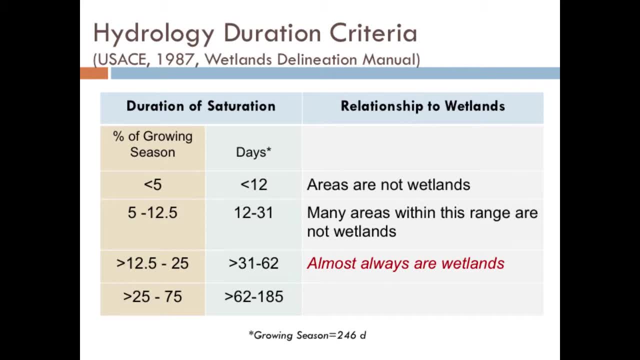 Well, if your duration of saturation within the critical depth is less than 12% of the growing season- less than 12 days, those areas are not wetlands. If it ranges from 5 to 12.5% of the growing season, roughly 12 to 31 days- many areas within this range are not wetlands. 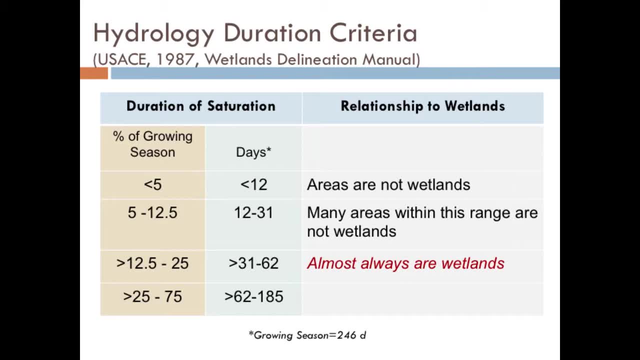 So what range do you want to use? So what type of duration criteria do you want to use? I would say you don't want to use anything less than 12.5%. If it's 12.5% or greater, almost all areas are going to be wetlands. 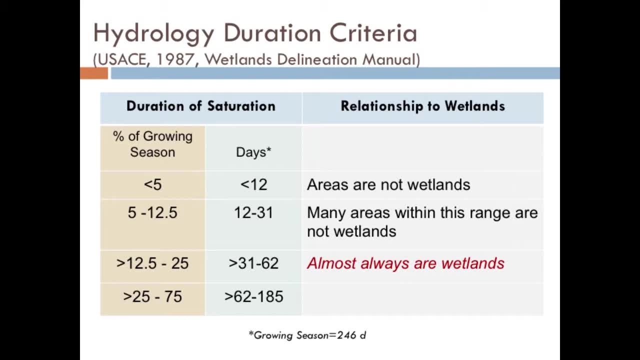 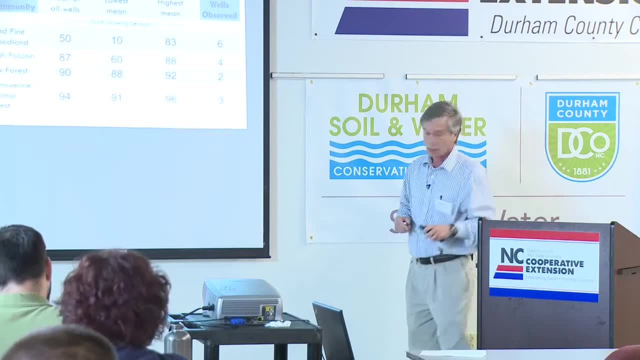 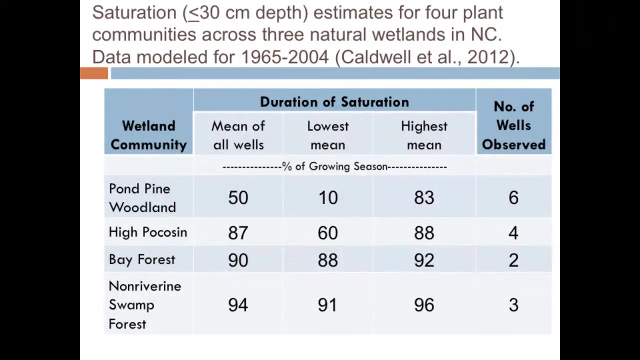 This is saturation in excess of 31 days. Anyway, that's what's in the core manual: 12.5%. Now we did some studies. a few years ago Our grad student, Pete Caldwell, said he looked at four natural wetland communities, some of which are used in restoration. 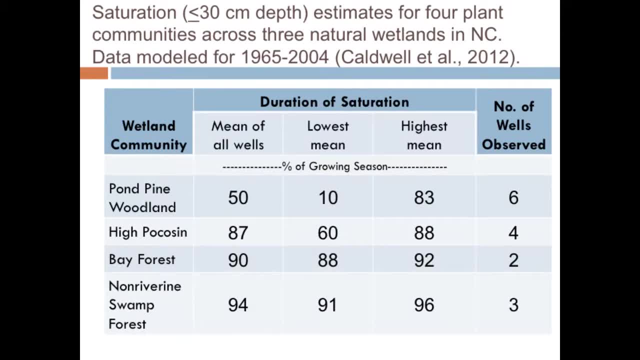 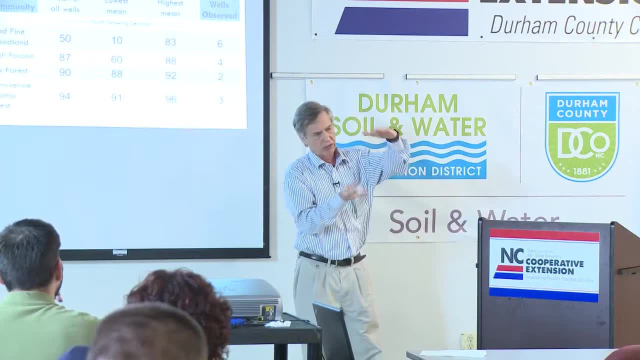 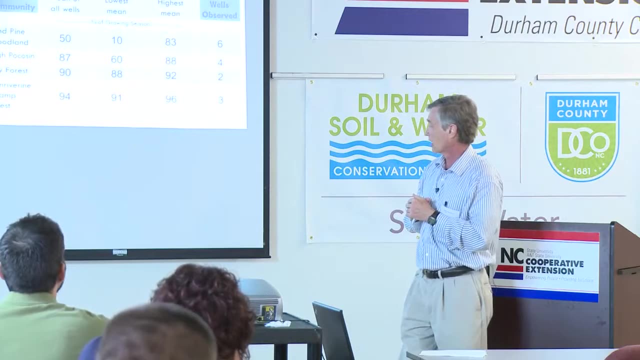 These are from three Carolina Bay wetlands. There are four plant communities, as shown here. And let me explain what he did. He looked at saturation within the top 30 centimeters of the soil. He went to the sites. I put a well into each of the plant communities. 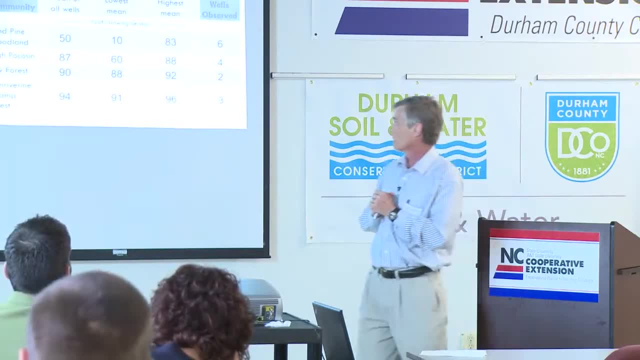 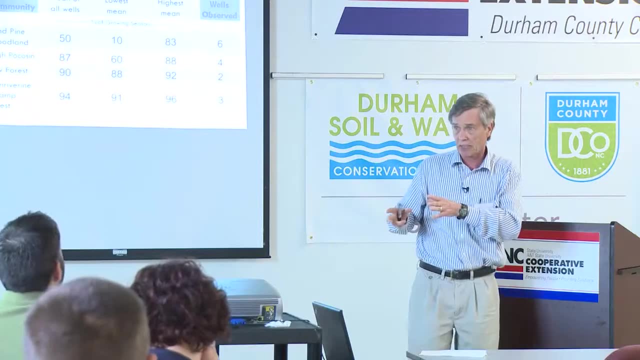 Usually they were replicated across the three wetlands. He then monitored them. He monitored water table levels for three years, took the data, calibrated a drain mod model for each well location That computes water table level when you plug in temperature and rainfall data. 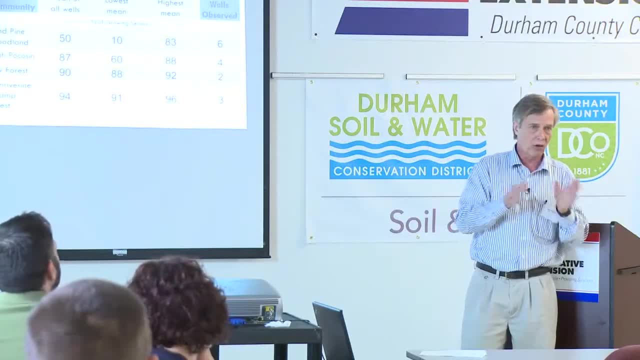 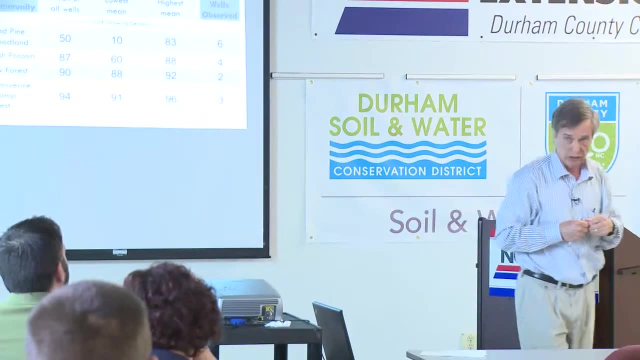 Then he went to the weather stations and got 40 years of daily rainfall and temperature data, plugged it into the drain mod model and calculated 40 years of water table data to get the wet and dry years. This is an average of his findings. 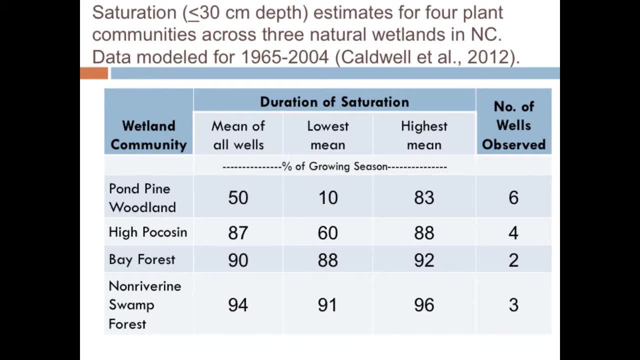 So these are the averages of his findings For a pond pine woodland. he found that if he averaged the 40-year data during the growing season now over all six wells, the pond pine woodland was saturated for 50% of the growing season. 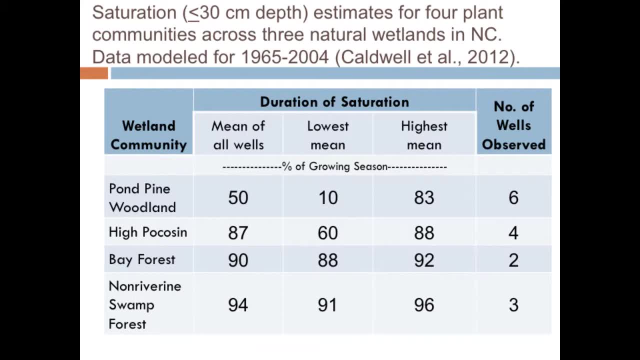 This is the frost-free period Now. across the six wells it ranged from a low of 10% to a high of 83%. For a high pocosin, you're saturated within the upper 30 centimeters for 87% of the growing season. Bay forest: 90%. non-riverine swamp forest: 94% over that 40-year period. The take-home message is: if you're going to use a duration of saturation of 12.5% based on these data, that is a pretty small duration to shoot for. 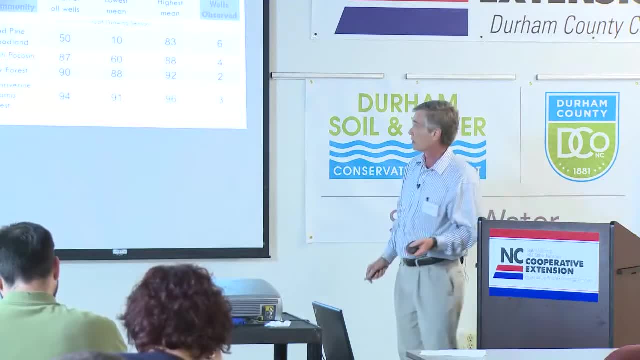 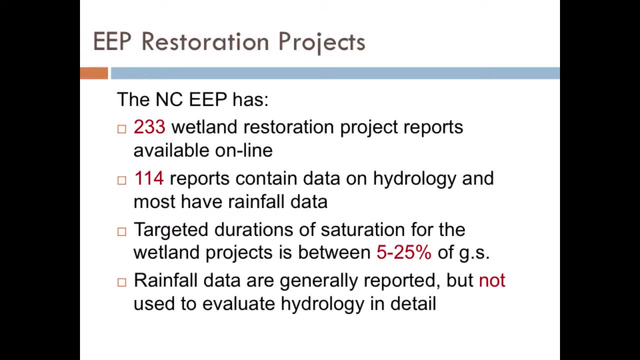 Our wetland communities are saturated for much longer periods of time, at least in these cases. Alright, let's take a look at the EEP's restoration projects. If you go to their website, you can see that they have reports for 233 wetland restoration projects online. 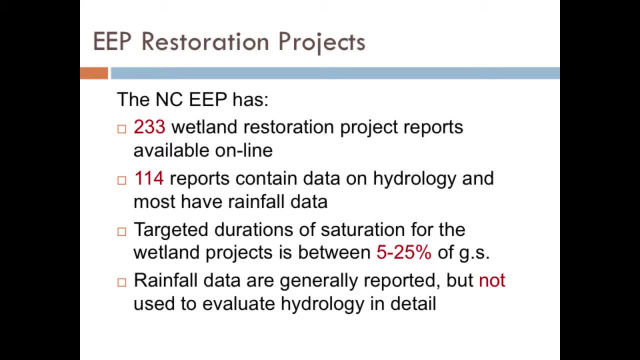 We selected 114 of those to look at a little closer because they have data on hydrology and rainfall. I'm not trying to imply that the remainder of the 233 are deficient in some ways, but usually they didn't have much monitoring data. 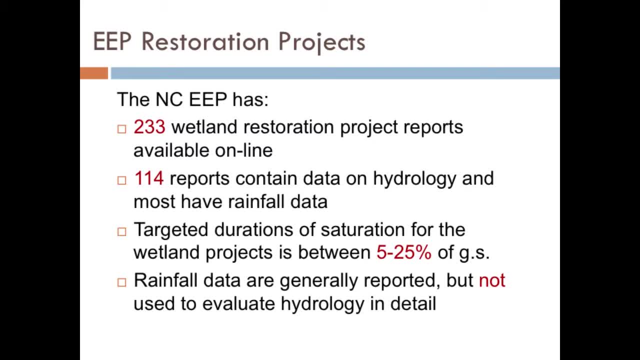 In other words, they only had it for maybe one year or were about to start, So we picked the 114 because they had multiple years. Just as a summary, the targeted durations used across all sites ranged from 5 to 25% of the growing season. 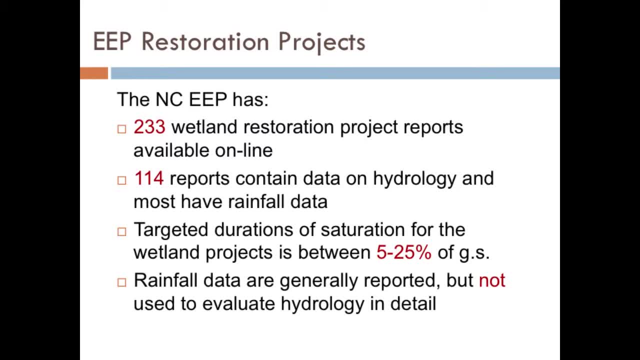 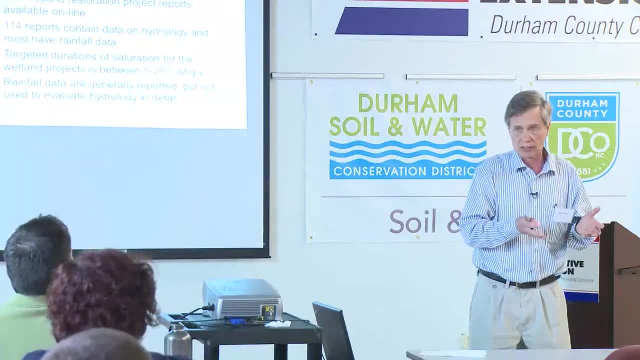 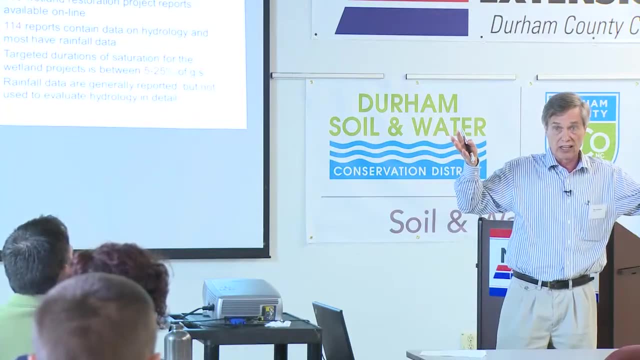 Rainfall data was generally reported but not used to evaluate hydrology in detail. In other words, if you have a wet year, normally the high water tables in the site do not count. If a hurricane comes through here, it raises the water table and we saturate a lot of land. 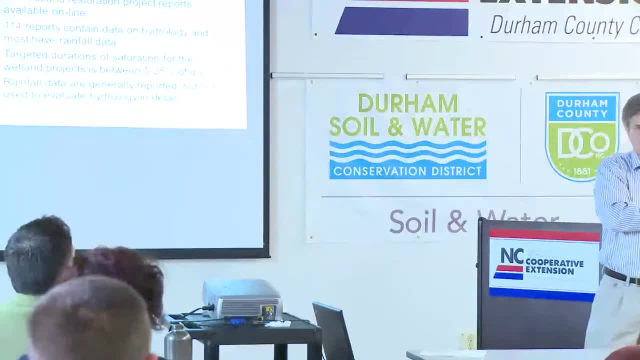 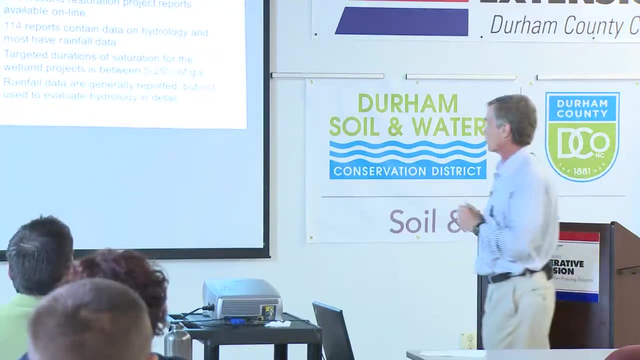 but not all of those are going to be wetlands, So you normally have to exclude data during wet collected durations, But in the EEP's data set it doesn't look like they do, possibly because there's not a standard procedure for doing it. 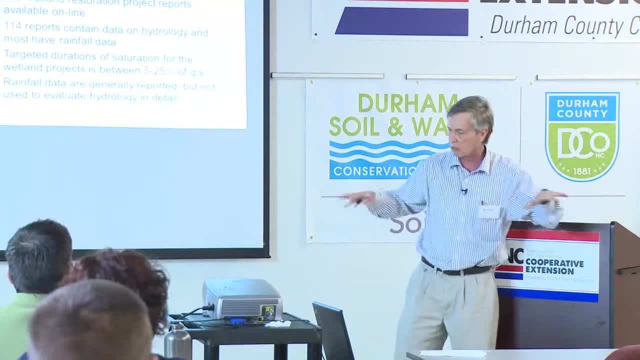 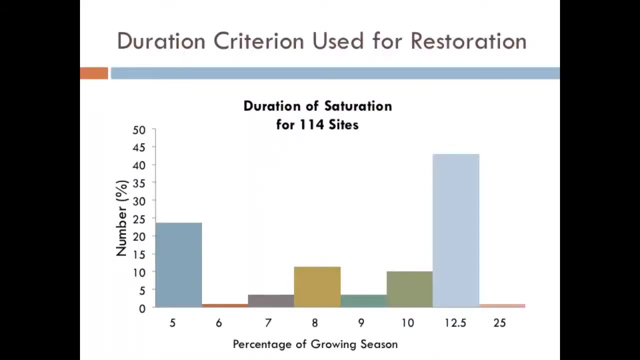 They report the rainfall data, they report the hydrology, but the two are never connected. This is the distribution of the durations of saturation for the 114 sites in the EEP's data set. You can see its duration is given as a percent of the growing season on the horizontal axis. 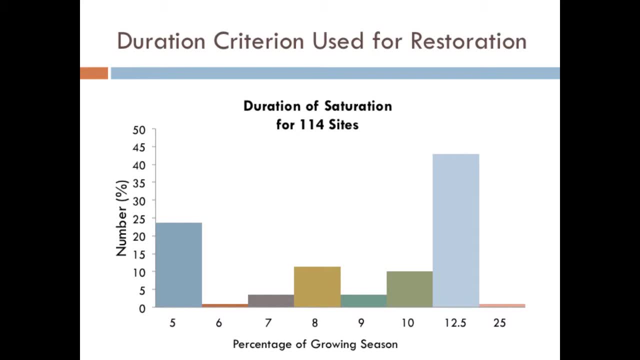 from 5 to 25%. Numbers as a percent of the total of 114 are on the y-axis, You can say that we had one site where the duration of saturation was 25%. That's a coastal area. So we're not discussing coastal areas today and only one of those sites again was reported. 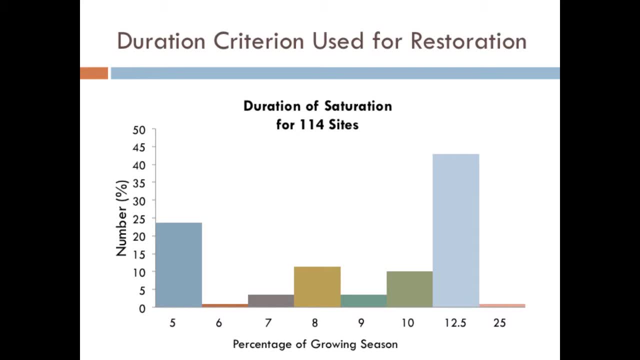 The most common duration used was 12.5% and that was found at about 45% of the sites. The remainder, about 50%, had durations ranging from 5 to 10%, with a fairly large number at 5.. Now I was just talking to Matt Hout and he said these are maybe the older sites. 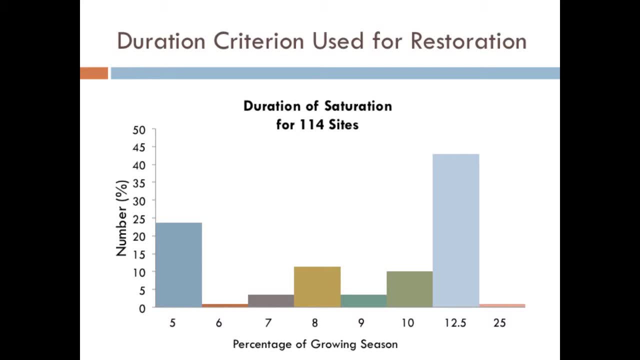 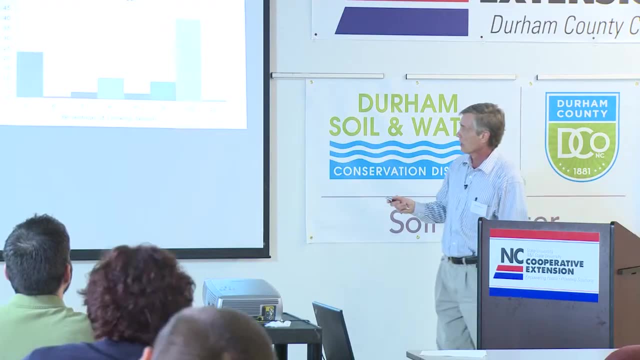 I'm not sure, But again, based on the Corps of Engineers criteria, this would barely be making the edge of a wetland for jurisdictional purposes. So the 12.5% looks like it's a little bit more appropriate to shoot for. 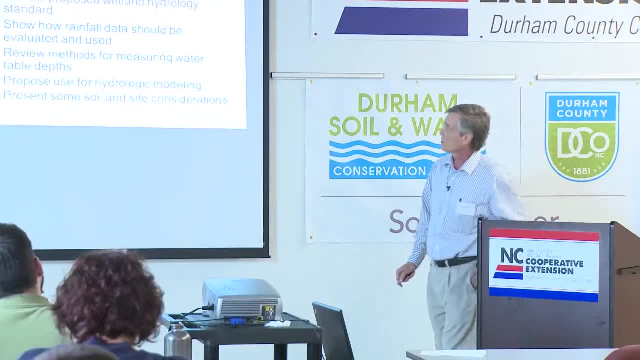 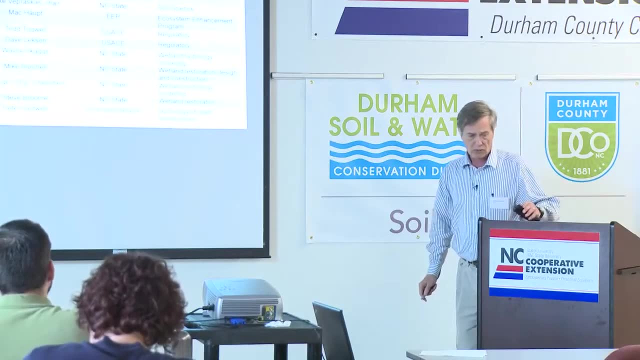 Okay, That was the first part of my objective. Let's turn to the second: our proposed wetland hydrology standard that we've suggested EEP use. Now, before I get into the actual guts of it, let me give you the committee. 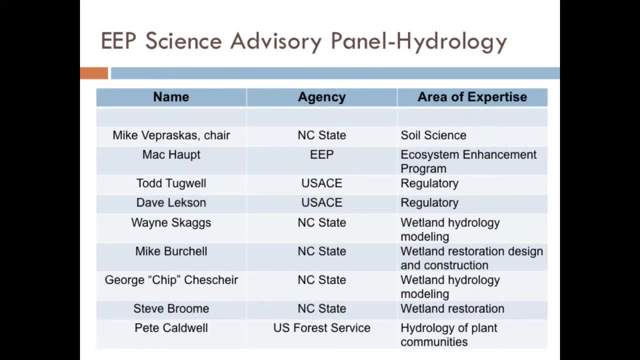 This is a subset or a subgroup of the science advisory panel and we were focusing on hydrology. I was the chair from NC State, Matt Hout, again from EEP. We had two representatives from the Corps of Engineers, Todd Tugwell, Dan Lexen. 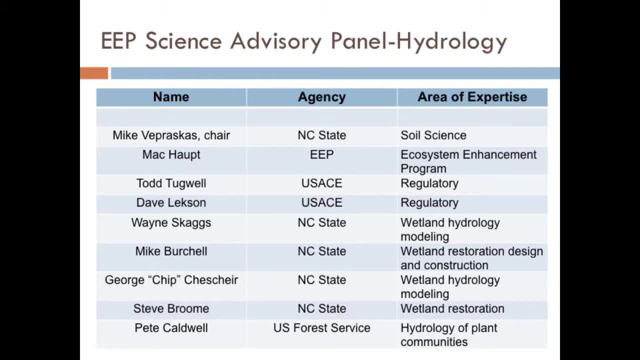 The next three guys: Wayne Skaggs, Mike Birchall, Chip, Cheshire, NC State engineers, hydrologists experienced in modeling and wetland restoration. Steve Broome at NC State, experienced with wetland restoration, And Pete Caldwell- I mentioned before- is with the Forest Service working on hydrology of plant communities. 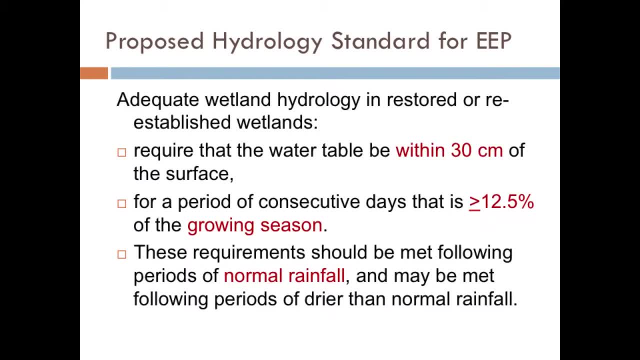 I thought it was a pretty good group. All right, Our requirements. the proposed requirements are as follows: Adequate wetland hydrology in a restored or reestablished wetland would require the water table to be within 30 centimeters of the surface. 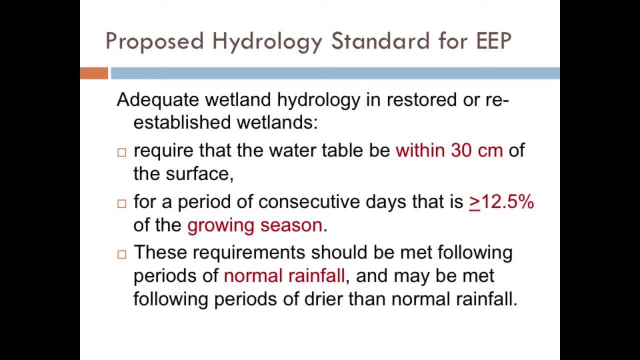 for a period of consecutive days greater than or equal to 12.5% of the growing season. These requirements should be met following periods of normal rainfall and may be met following periods of drier than normal rainfall, But the point is, you would be meeting these requirements during a period of wetter than normal rainfall. 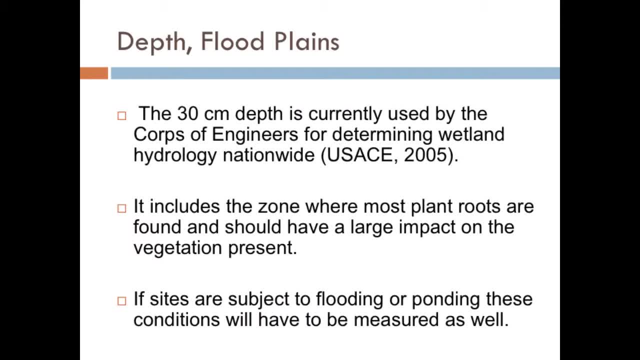 would be considered unacceptable. Now, the 30 centimeter depth requirement, of course, was taken from the Corps of Engineers. This is a zone where a lot of your roots will be found, and so saturation in this zone should affect the plant community. 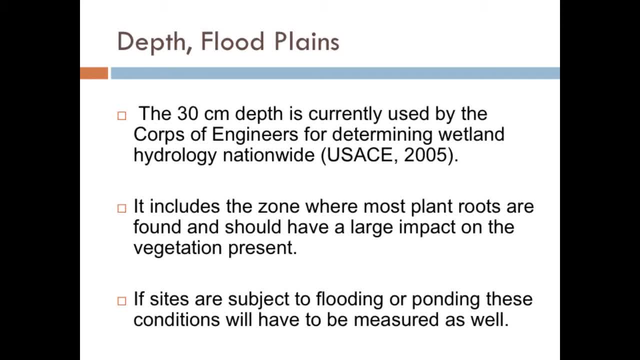 We did not consider sites subject to flooding or ponding at this time. Maybe this can be brought in. We focused strictly on the water tables, But if flooding and ponding are occurring, you'd want measurements of those as well. I didn't mention anything about duration. 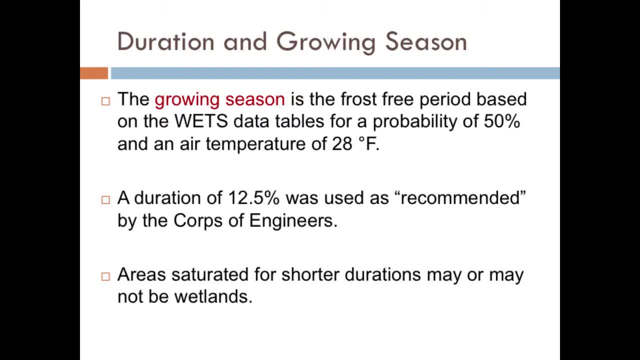 so let me put it in. I did mention duration, but let me talk about growing season. related to that, The growing season is what is? the growing season is being debated somewhat in North Carolina. Some people feel it's year-round, based on soil temperatures. 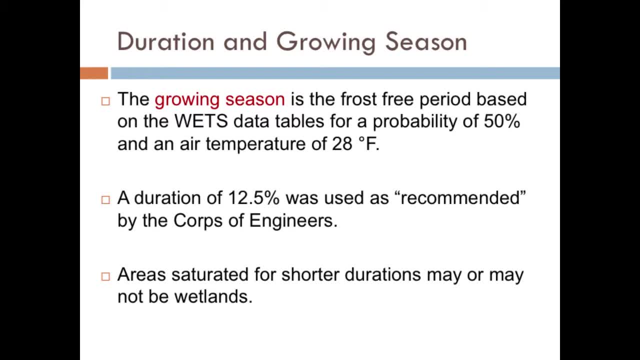 For this criteria. we want to use the frost-free period for the growing season and that's available on the dates of that are available on the wet data tables online. Use a probability of 50% and an air temperature of 28 degrees Fahrenheit. 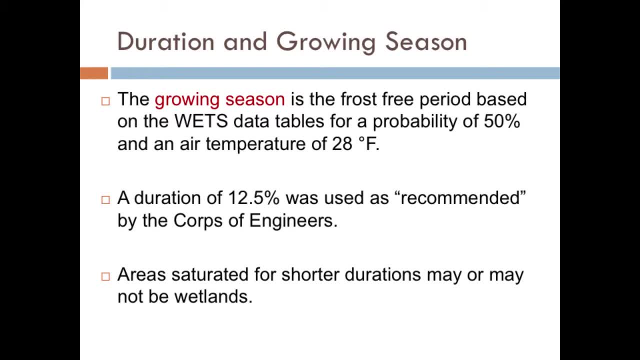 Now, who has heard of the WETS data tables? Okay, most of you, and so you know where to go and you'll be able to get it. I'll show an example a little bit later. A duration of 12.5% was selected as recommended by the Corps of Engineers, primarily. 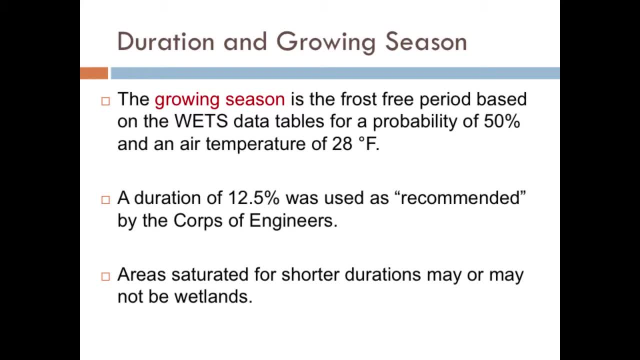 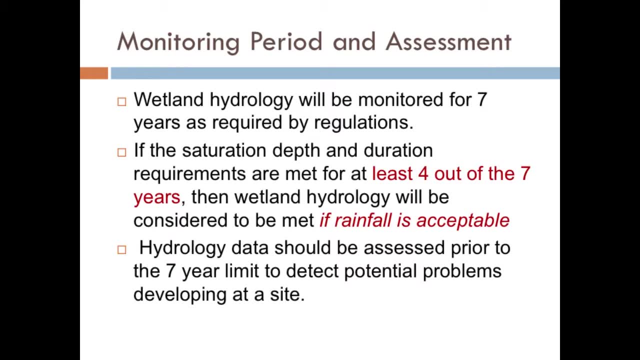 Areas with shorter durations may or may not be wetlands, based on the information I showed you earlier. Okay, monitoring. This goes back to frequency, or will include frequency? We're recommending, at least according to math, that wetland regulations will require. 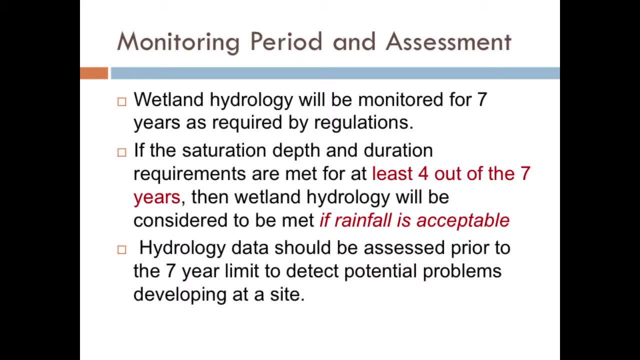 if they don't now that monitoring be done for seven years. That's not my rule, That was handed down to us And we're saying that the saturation depth and duration requirements are met for at least four out of those seven years, During periods of four out of seven years. 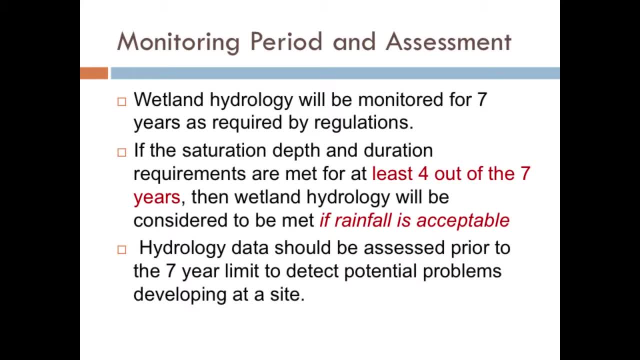 the hydrology will be considered met if rainfall is acceptable. Okay, So you've still got to use rainfall And we recommend that assessing hydrology annually just to see if there's problems developing at your site, because if you find that it might be a little dry. 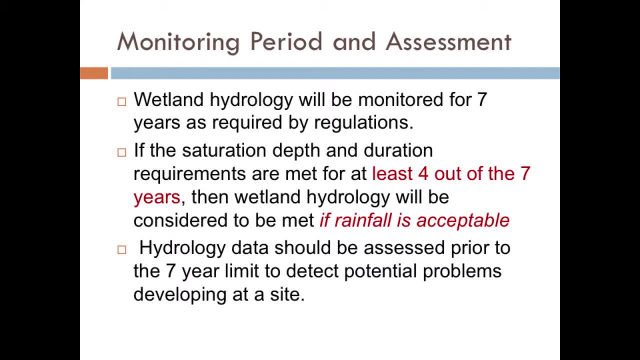 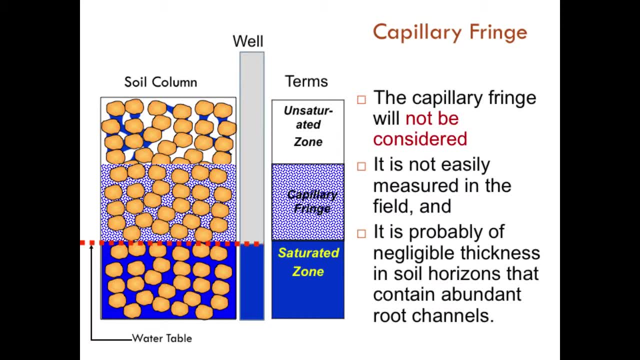 there still might be time to make modifications to increase the water table elevation. I don't know if those of you who are familiar are worried about the capillary fringe, but if you deal with wetland regulations and hydrology, this issue always comes up. 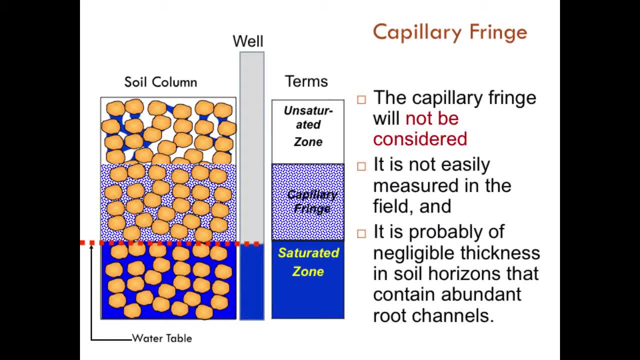 If you don't care about the capillary fringe, that's fine, because our recommendation is: don't worry about it. Now let me explain why. We've got a soil column over here on the left with three distinct zones. We've got a well here with the water level. 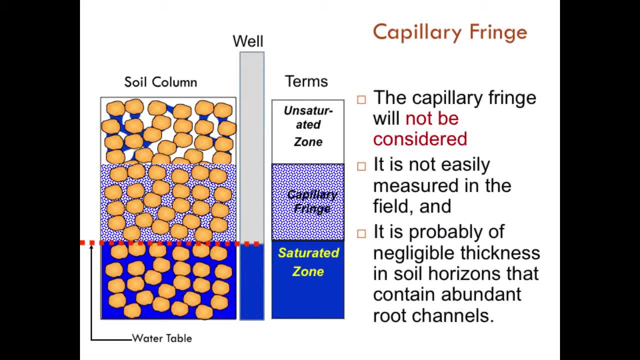 shown by the dashed line, And then I've given names to each of these three zones. So we've got the saturated zone, the capillary fringe and the unsaturated zone. Here's my water table. You can see that it equals the water level in the well. 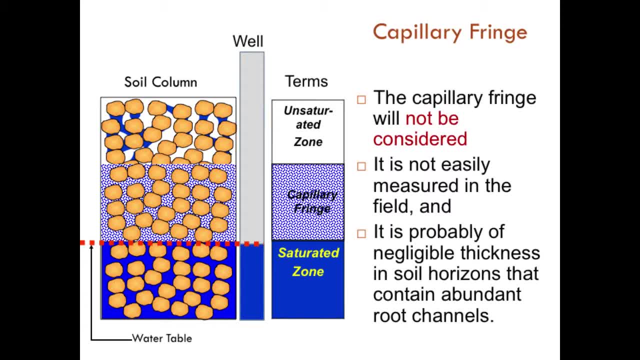 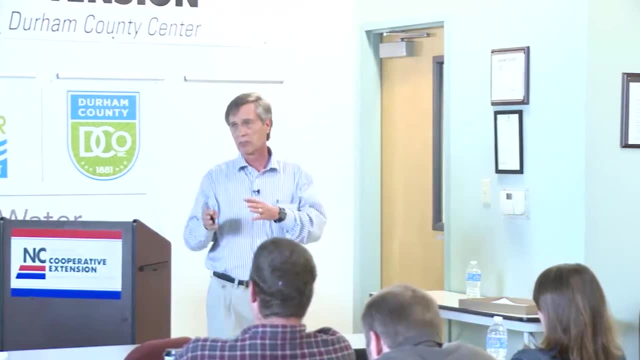 Now below it, in the saturated zone below the water table, the pores are full of water and the water has a pressure greater than atmospheric pressure. Need I say more? Now let me ask you something. Is that an academic definition? the pressure on the water is greater than atmospheric. 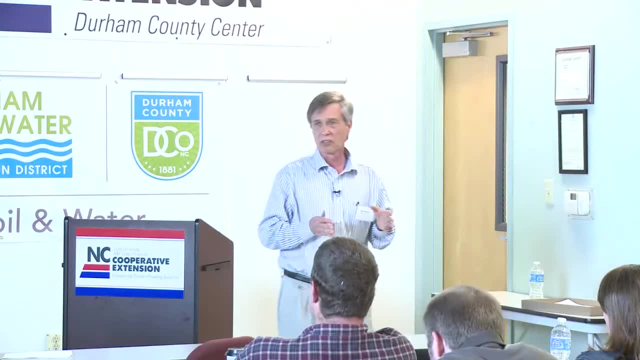 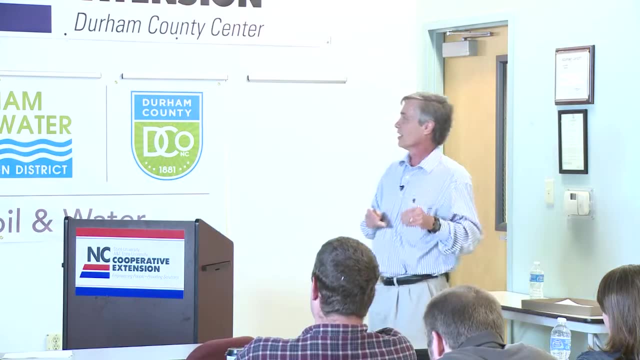 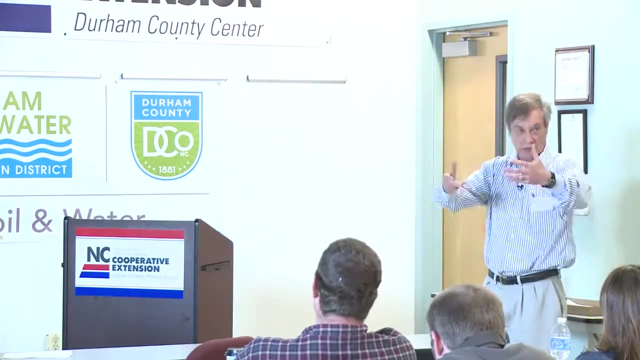 or is that field-friendly? Could that ever be used? What do you think? Okay, Let me explain this. When the water has a pressure greater than atmospheric, we call it free water. It flows by gravity as well, But it can enter a well. 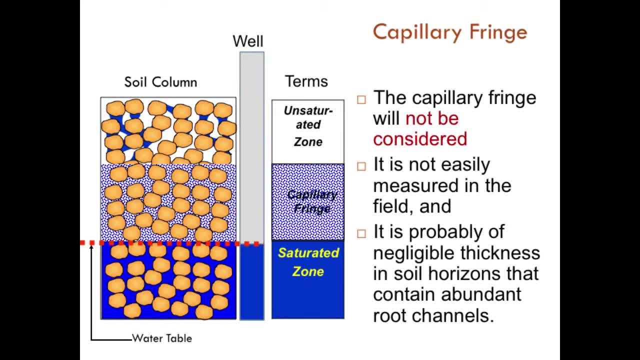 because it can push air out of the well. So it is a field-friendly definition To know when the water has a pressure greater than or equal atmospheric. look at a well, a borehole or a ditch. If there's water in that ditch. 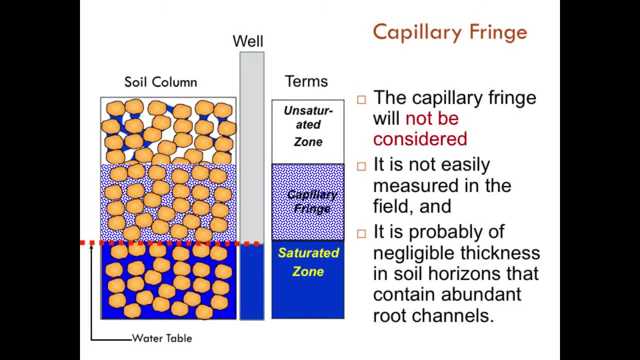 that surrounding area has water with a pressure greater than atmospheric. It's field-friendly. Now, why do I say that? Old academics standing up here? Well, that's a saturated zone. Now above it we have the capillary fringe. Again, all pores are full of water. 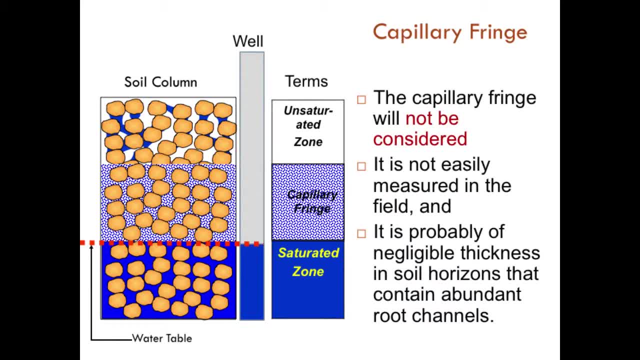 but here the water is held under a tension or a suction. The pressure is less than atmospheric. So what does that mean? It cannot flow into a well. It cannot push air out of the way As a result, when you're using wells or piezometers. 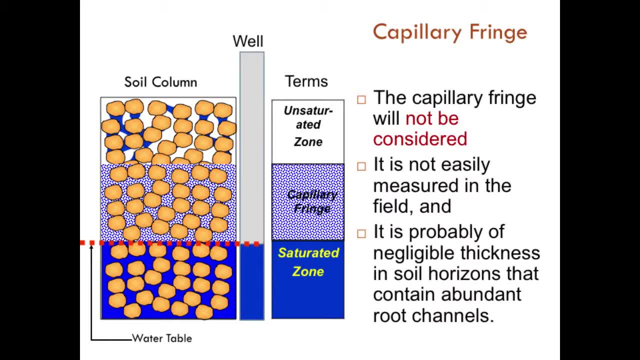 you have no idea how thick this zone is, So I say you forget it. The true unsaturated zone where the pores are full of water and air is above this. So the capillary fringe is something we're not considering. It's not easily measured in the field. 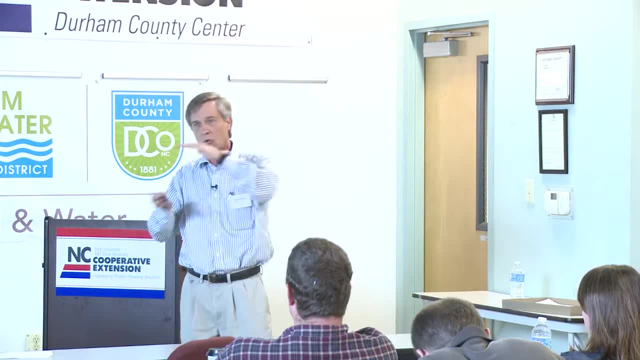 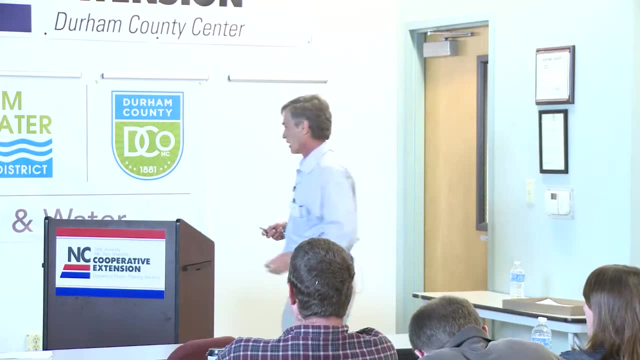 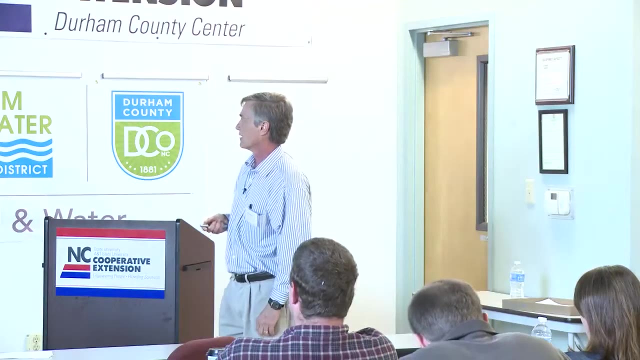 My personal opinion is that if we cannot measure it, we cannot require it in regulations. Okay, Otherwise you're dealing with somebody's opinion, Something like an academic. We sure don't want that for regulators. And it's also of negligible thickness in soil horizons that contain abundant root channels. In other words, if you've got root channels one to two millimeters in diameter reaching the water table, that is too big for them. They're too big to suck up much water, to draw water up, And so the capillary fringe in the rooting zone. 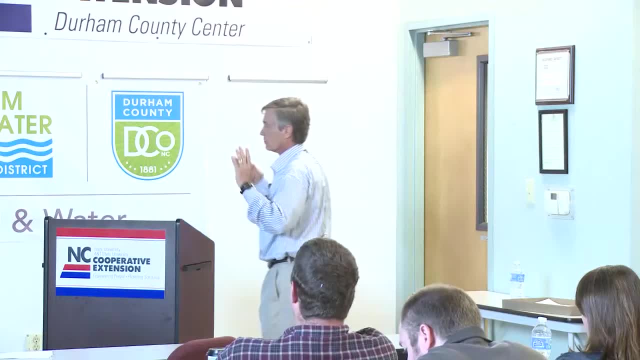 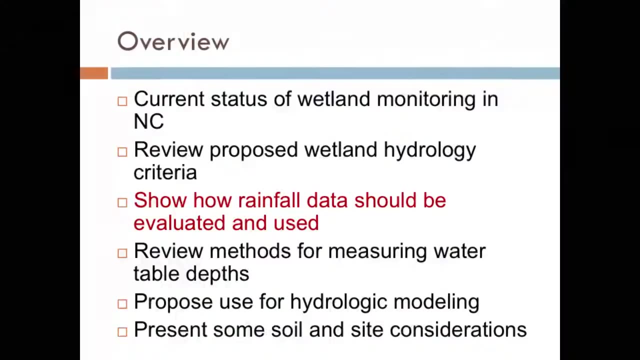 is probably going to be very, very thin, All right, And virtually irrelevant, So forget your capillary fringe. Ah, my favorite topic, rainfall. Let's talk about how rainfall data can be interpreted, because this might be a little on the odd side. 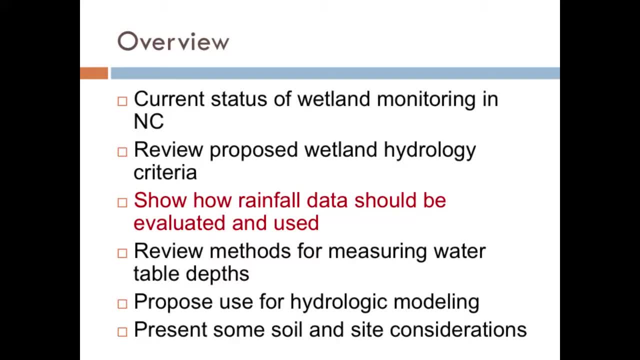 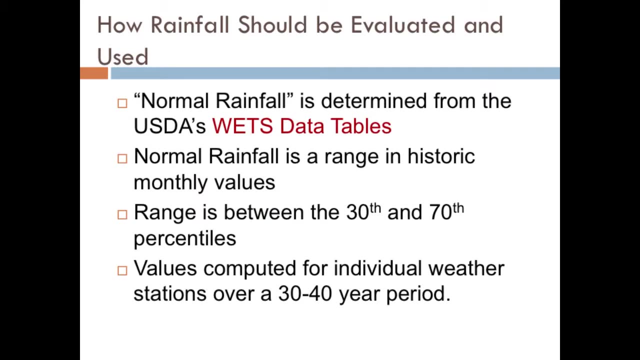 or new for you. Now we're using the term normal rainfall condition: wetter than normal. drier than normal. The normal rainfall is going to be defined on the USDA's wet data tables. We're using those as our definition of normality. 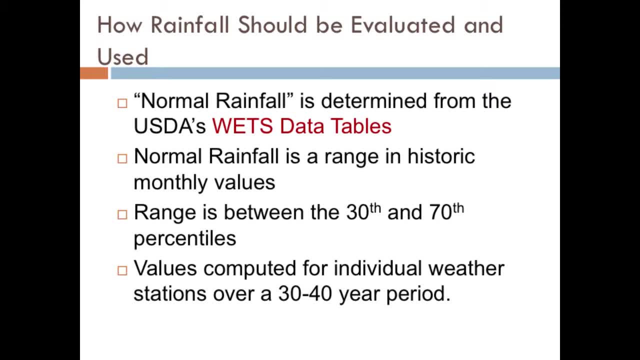 Normal rainfall is given as a range of rainfall values. on those tables It's defined as the 30th and 70th percentiles, And these values are computed over a 30- to 40-year period. I'm looking out at your faces right now. 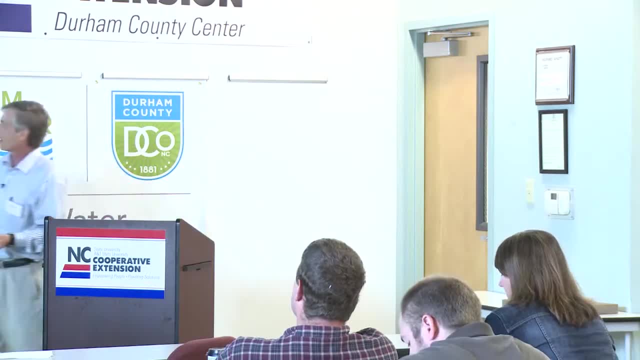 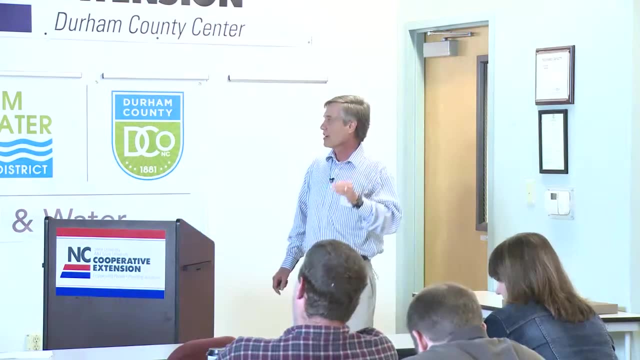 and I see you're ready for more. You're eating this up. So, okay, I'm not going to hold back, I'm going to unload. Believe it or not, this is kind of interesting. Now, if you want the WETS data, it's available online. 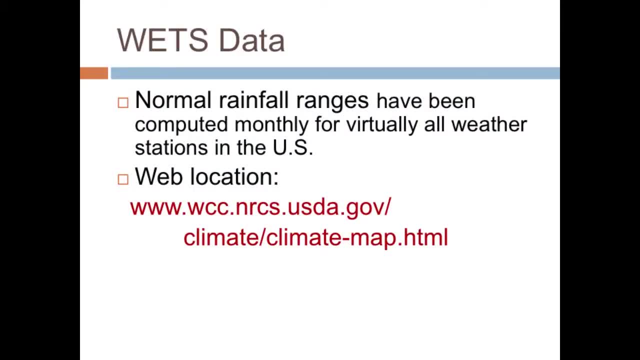 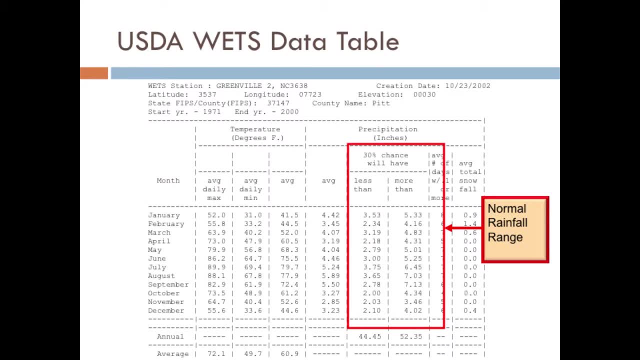 I checked this out last week so the website is still valid, I hope. Now here's a WETS data table. I hope you can see the numbers. If not, the one in the book looks pretty good. This is for Greenville, North Carolina. 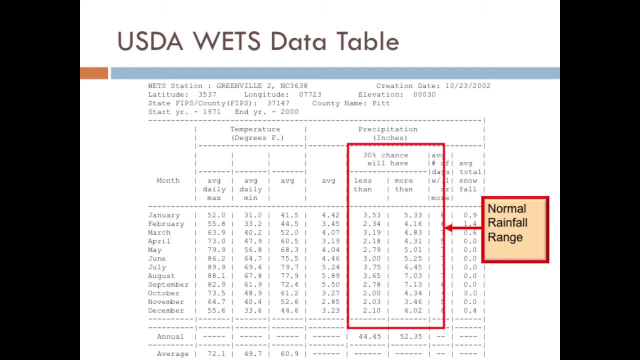 You can see in the first column we've got months: January through December. The next three columns are temperature. We can cross those out. The last five columns relate to precipitation. Now we have a column here with average precipitation. If you scratch that out, we don't care. 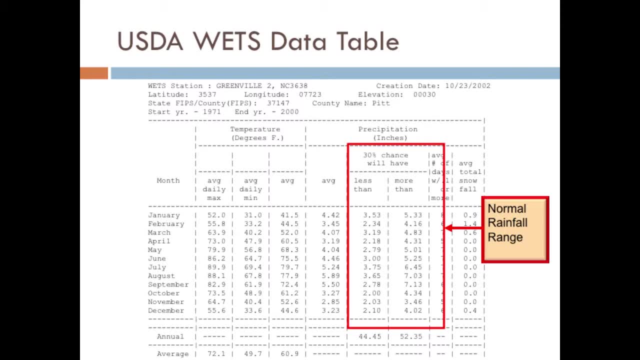 It's the next two columns that we're interested in. These are the 30th percentile and the 70th percentile. Okay, so basically this is the 30th percentile. It says 30% chance we'll have less than this amount. and there's a 30% chance you'll have more than this. This is our 70th percentile, So our normal rainfall range at Greenville for the month of January is 3.53 to 5.33 inches of water. Any questions on this? 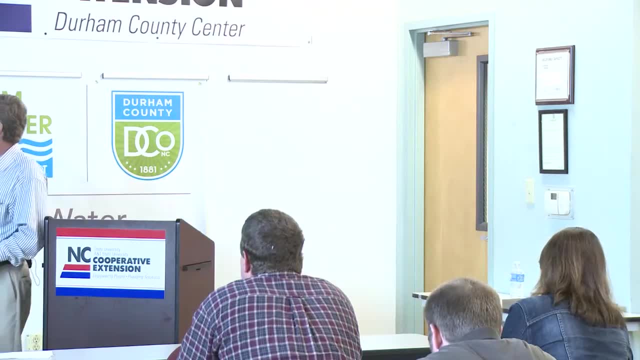 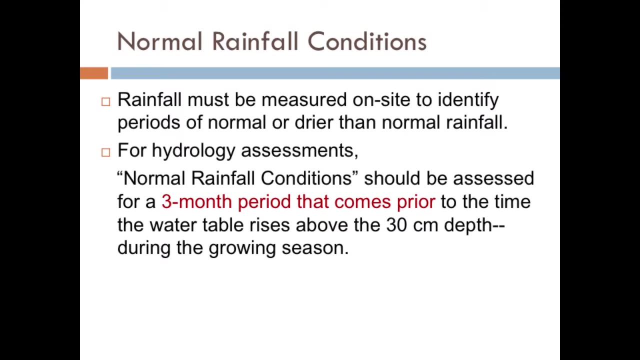 Very simple: Anything above that is wetter, Anything below that range is drier. Okay, Now we are recommending that rainfall be measured on site to identify periods of normal and drier than normal rainfall for the hydrology assessments. Now for those assessments. 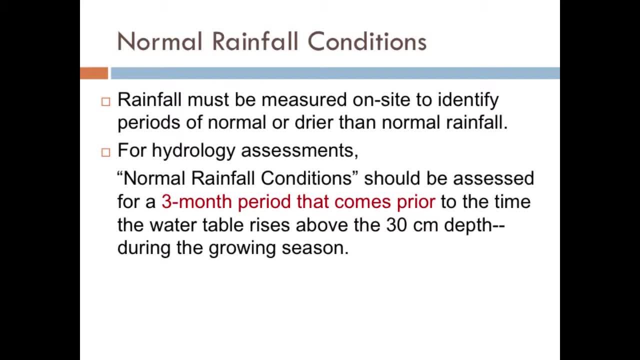 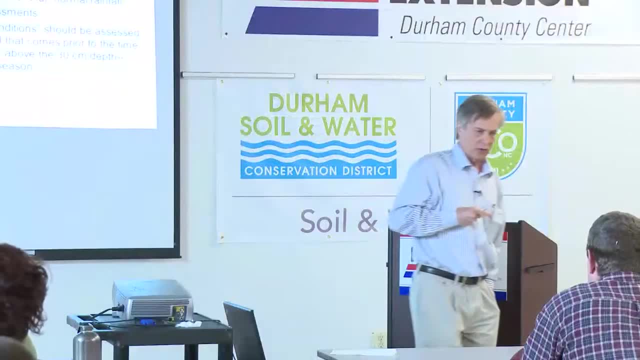 the normal rainfall conditions should be assessed for a three month period that comes prior to the time the water table rises. That struck me when I first heard it as a little odd. I would have thought you'd want to measure rainfall or look at your rainfall. 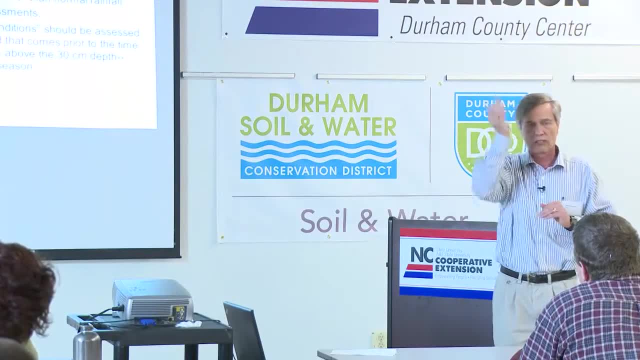 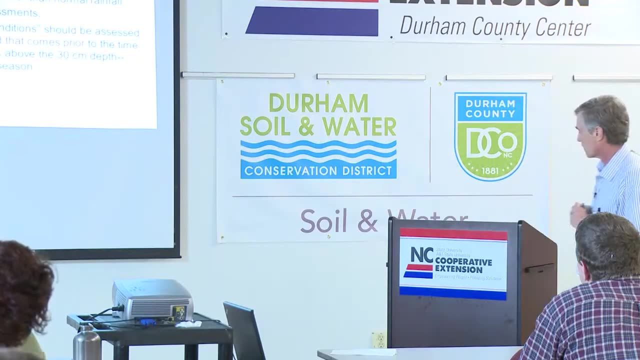 after the water table rose. But no, the Corps of Engineers has recommended that you look at it before the water table rises, and we're recommending a three month period be examined. Now let me show you what I'm talking about. All right, 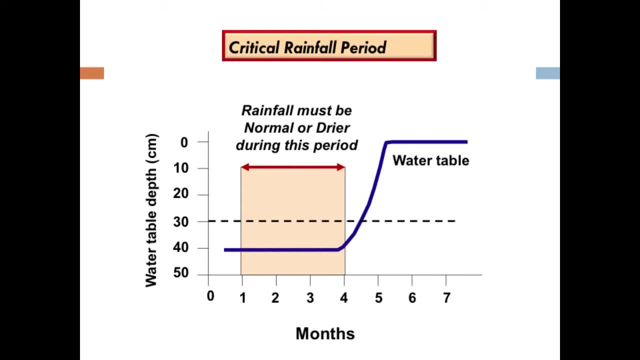 Here is a diagram. We just made this up, so let's see if we can work through it. This is a graph of water table fluctuation over time. So here's months of the year and you can label this January, February, March, April, whatever. 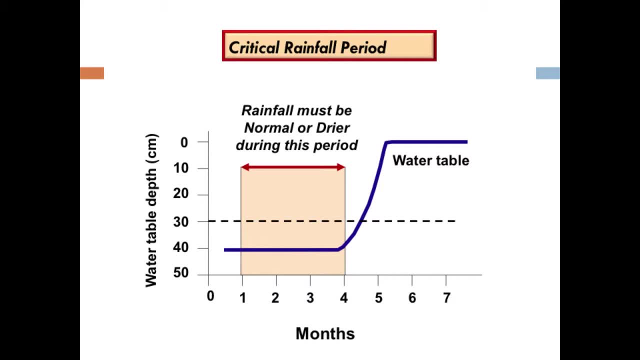 For this area, the growing season is somewhere in month, about midway through month three, And you can see here this is the depth from the soil surface. In January, February, March or whatever, the water table is below the critical 30 centimeter depth. 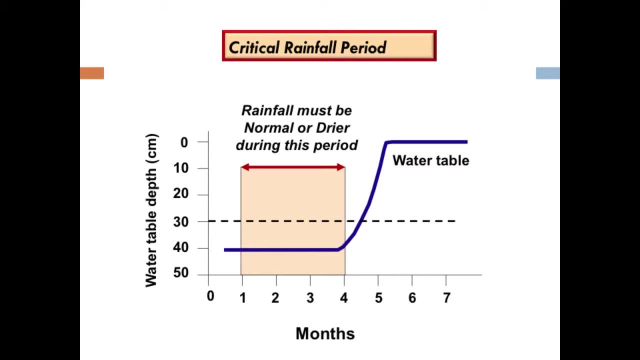 But in month four it kicks up to the soil surface and remains there for several months. So the water table rose during the growing season and stayed above 30 centimeters for several months. We've got the depth, the criterion met, the duration is met. 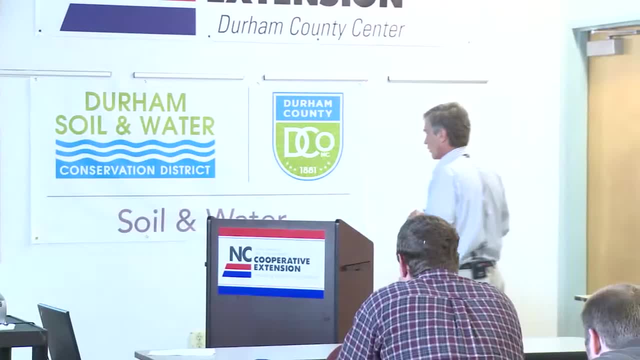 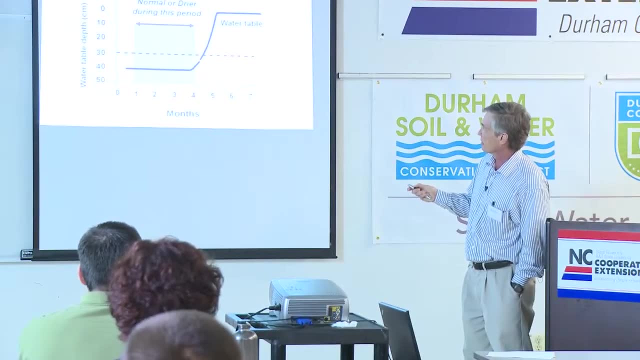 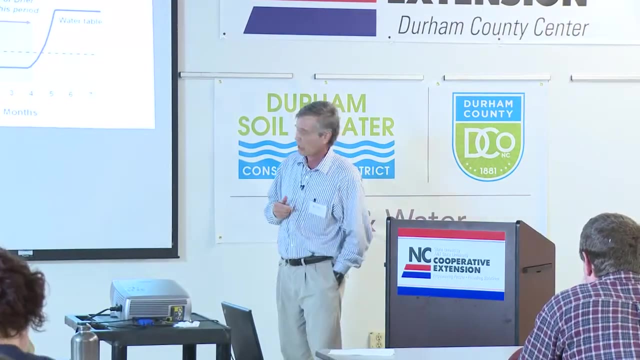 but did this occur during a period of normal or drier than normal rainfall? To answer that question, you consider the rainfall during the three month period prior to the time the water table rose. This is basically a policy of the Corps of Engineers or a recommendation from the Corps of Engineers. 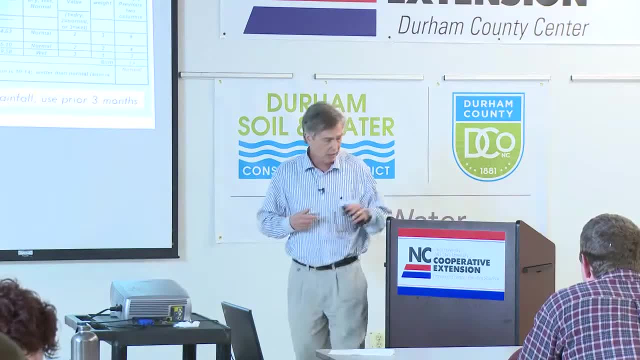 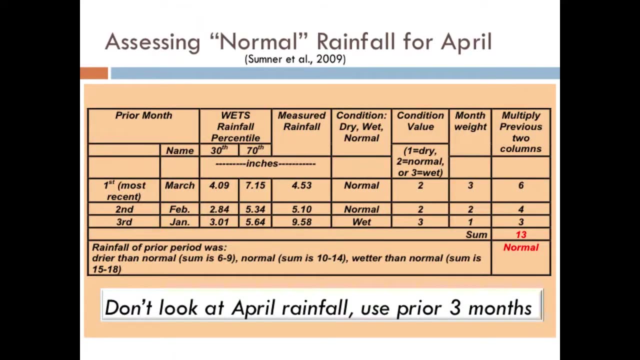 in the Rainfall Assessment Guidebook. Let's walk through a table that makes rainfall evaluation quite simple. Let's say, the water table rose in April And, by the way, the method is also published in a study by Sumner, a student at NC State that worked with us. 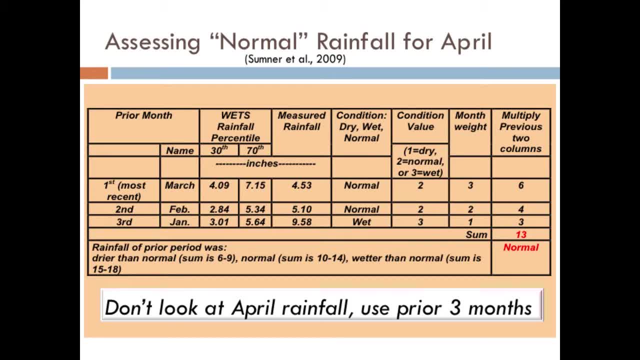 She's compared several rainfall assessment techniques studied by the Corps or proposed by the Corps of Engineers, And this one turns out to be the simplest and one of the more accurate ones, actually. So you start with a table like this: Water table rose in April. 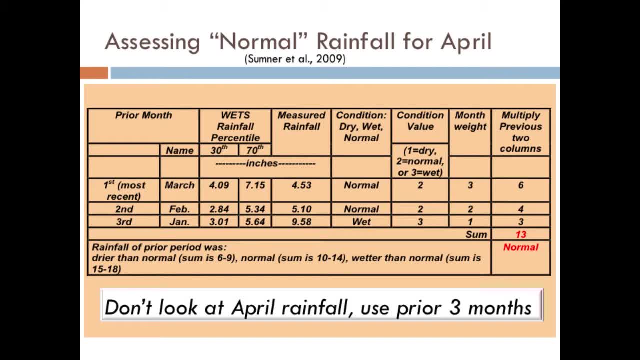 So in this table you have to first list the months of interest. The prior three months are March, February and January. Alright, Next two columns. you put your WETS data. So this is the 30th percentile column. 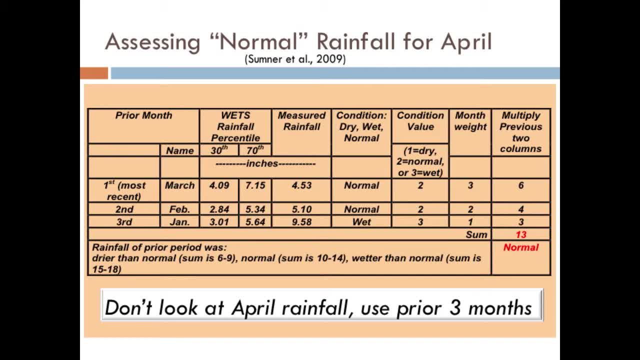 and the 70th percentile column. Then this column shows your measured rainfall determined on site 4.53,, 5.10, 9.58.. You fill that in. Then you put a condition on it: that rainfall. 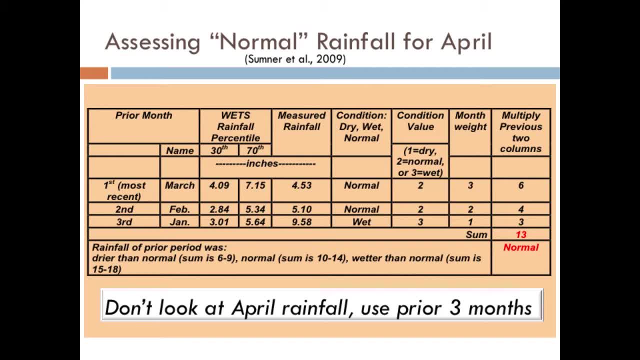 So in other words, 4.53 is in between the 30th and 70th. This is normal rainfall, 5.10 in between normal, But 9.58 is well above the 70th percentile, and so this is considered wet. 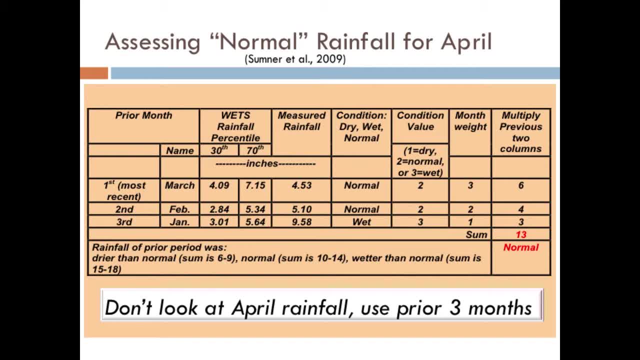 Alright, And wet rainfall might still be usable. but you just have to run it through this table to be sure. After you've got the condition, you put a condition value: 2 for normal, 3 for wet, 1 for dry. 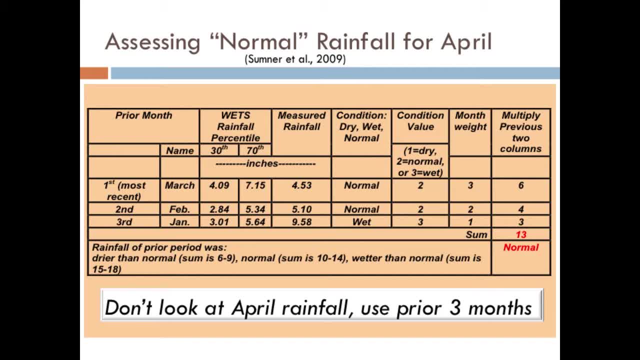 So you've got 2,, 2, and 3.. You have a monthly weight: 3,, 2,, 1.. And the last step: you just multiply these two columns together. 2 times 3 is 6.. 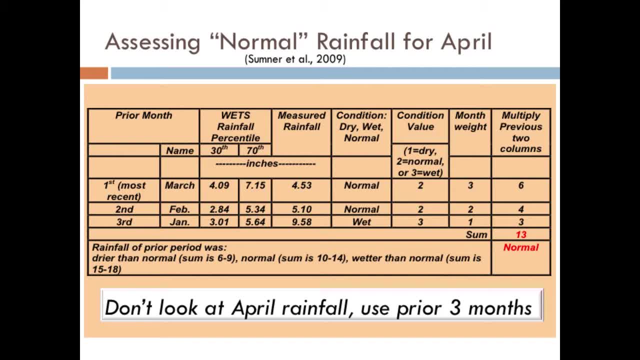 2 times 2 is 4.. 3 times 1 is 3.. Add them up to 13. And that's the number you use. You come down here and it says: normal is where your sums are between 10 to 14.. 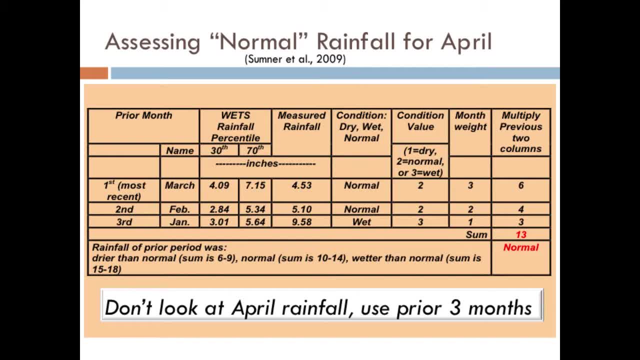 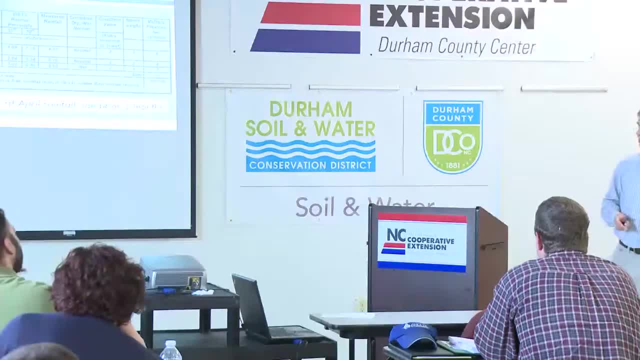 So in this case, the rainfall is considered normal for a three-month period. Alright, Very simple technique to use. I could give a test right now and you'd be able to go through this Any questions? Yeah, So, Mike, you start. 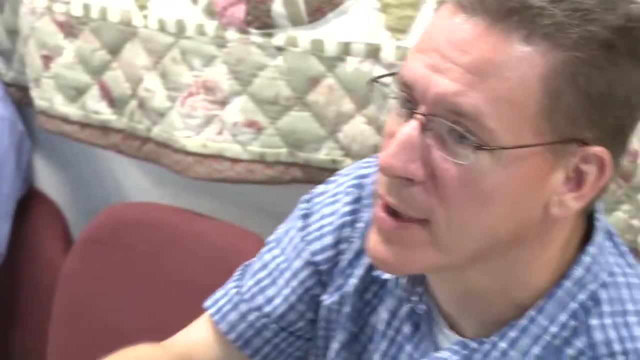 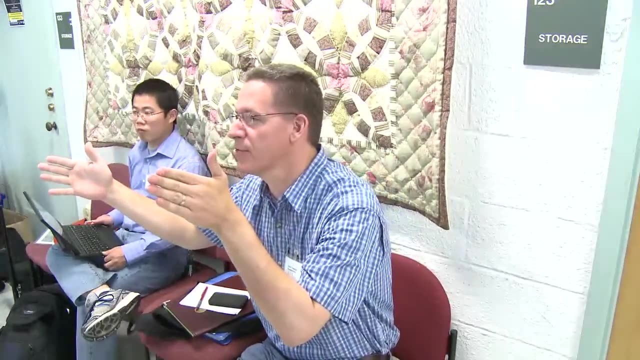 you would start that three-month analysis at the point where you- your water table rose and you had a period of whatever that you felt like you met your criteria or you did meet your criteria. You were above 30 centimeters per month. That's right. 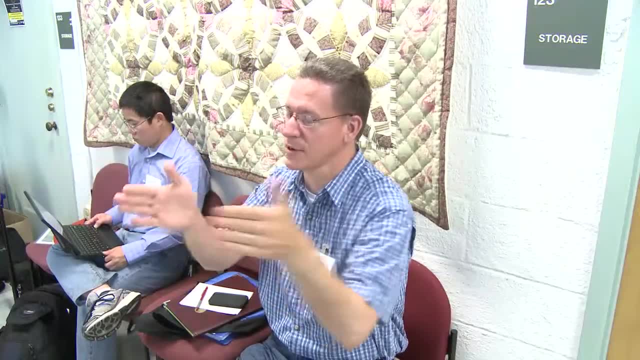 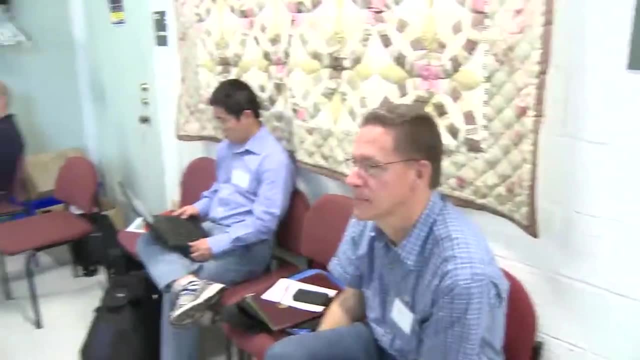 So if you want to see if that is a usable set of data, you would look at the three months prior. That's correct, Right? So you can't just report the water table data. You have to make sure that the rainfall. 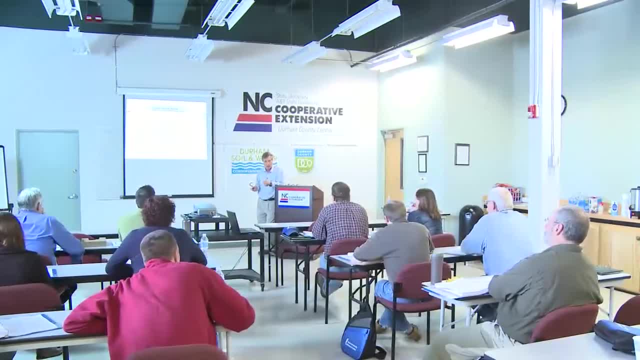 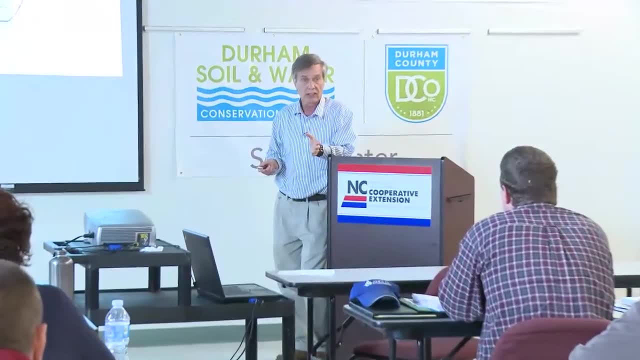 that created that high water table was either normal or drier than normal. Okay, So some of the water table data that will be collected by you guys will have to be excluded or not used in assessing wetland hydrology by this recommendation. Yeah, Neil. 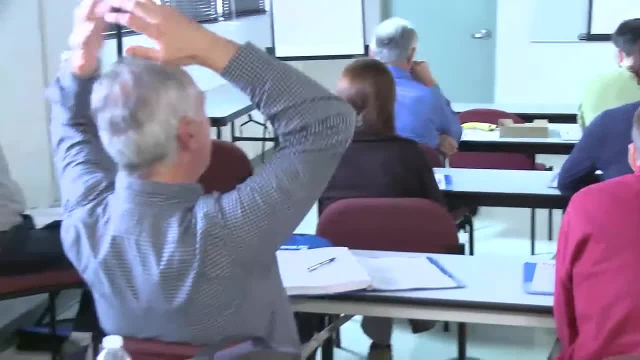 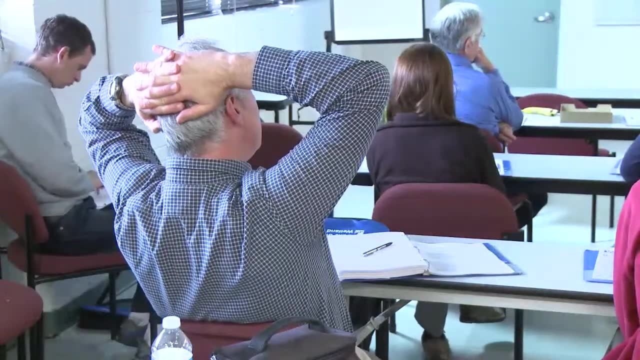 So just in planning your assessment, would you then typically plan on doing 10 years of monitoring and get seven valid years? Not necessarily. It depends on how. I think it depends on the success of your site. I mean if you have built the site. 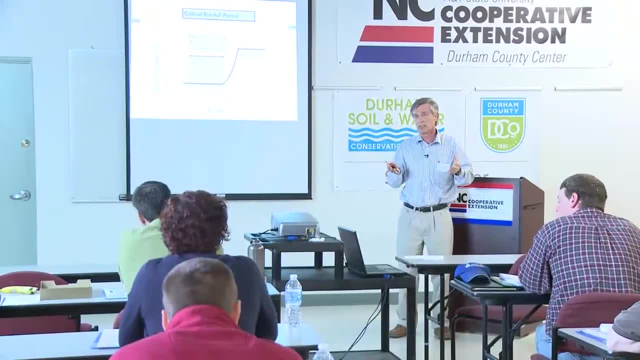 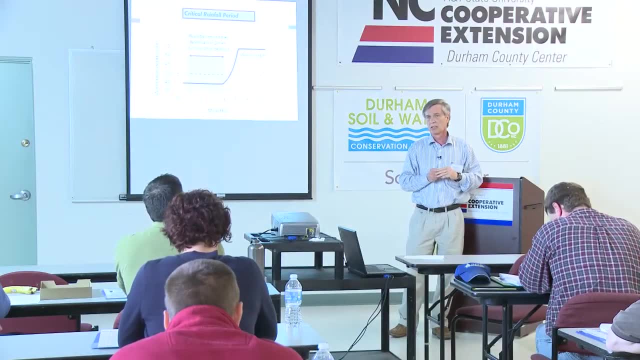 or restored the site to be wet enough. you don't need 10 years of data, All right, So I don't necessarily think this is an unusually difficult standard to meet. Yeah, What made you choose three months over the start of the day? 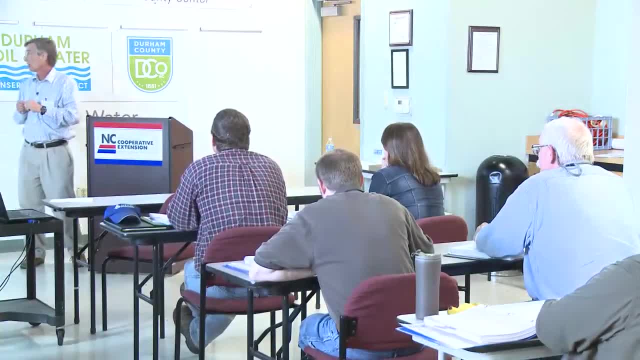 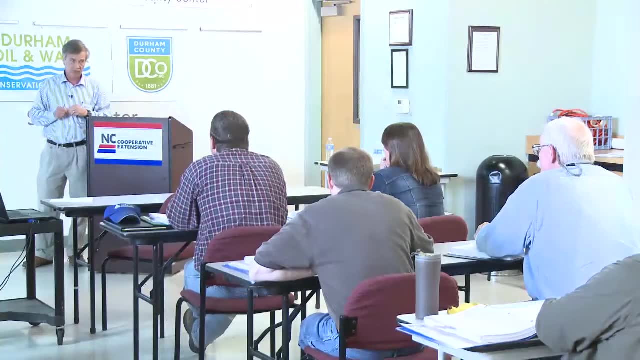 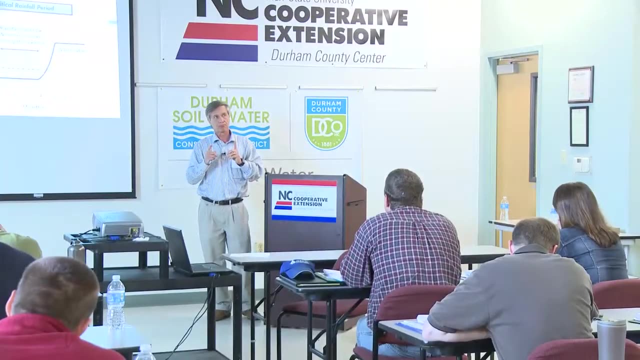 to find out prior to one month start. Well, a couple of reasons. One: the Corps of Engineers recommends, I think, four different methods for evaluating rainfall. This was one We did look at a shorter period, including periods over the. 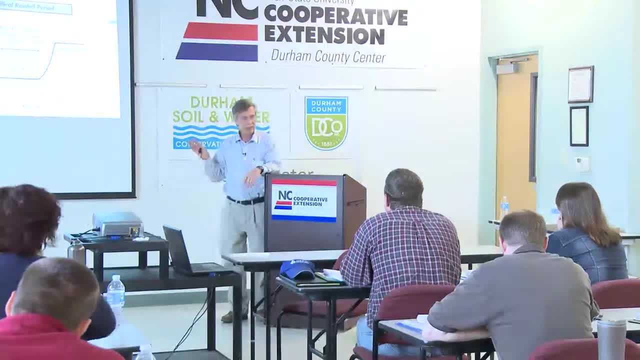 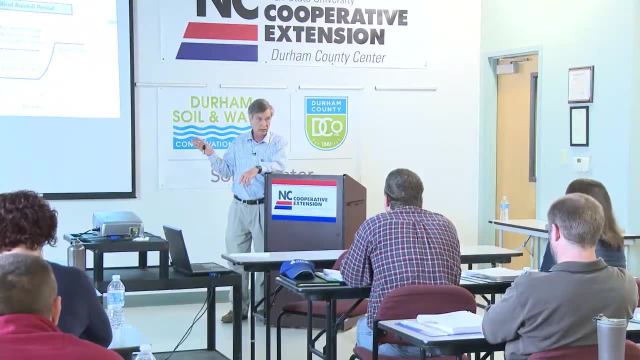 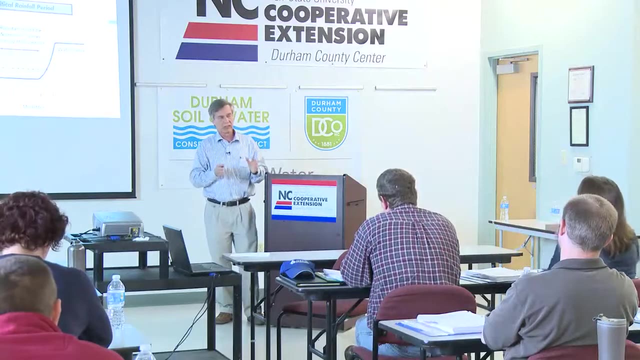 after the water table rose, And this method turned out to be one of the better ones. Okay, So we tested it and it worked as the answer. Okay, well, all right, we went to a site that was a wetland. 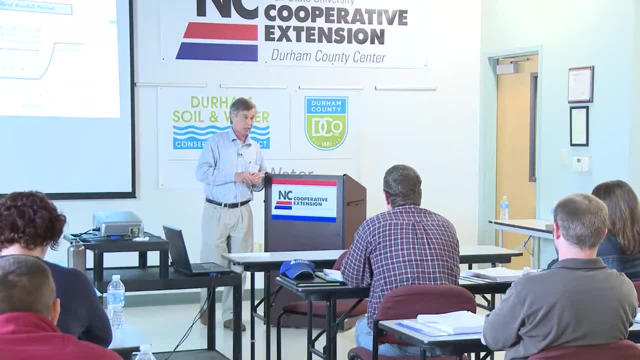 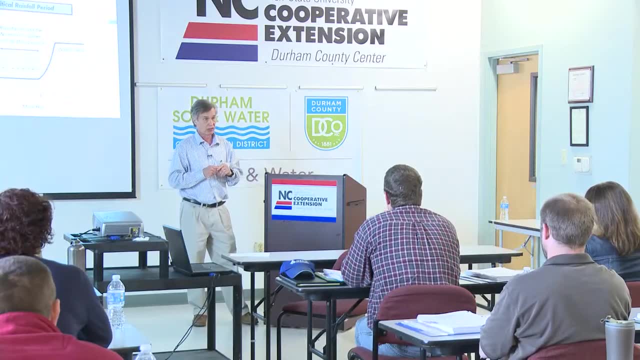 and it was on the wet. it was a range and so it was saturating. I think it had a water table within 30 centimeters for 95% of the years- Okay Nine out of 10 years- it meets wetland hydrology requirements. 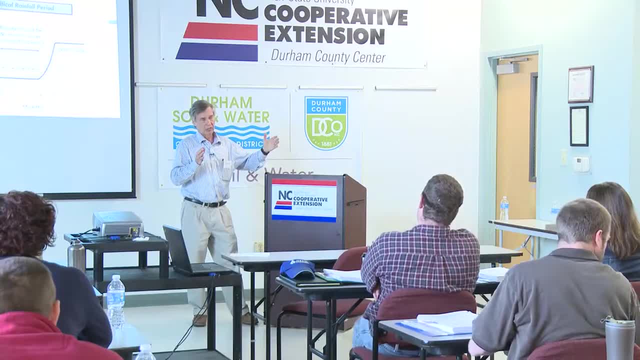 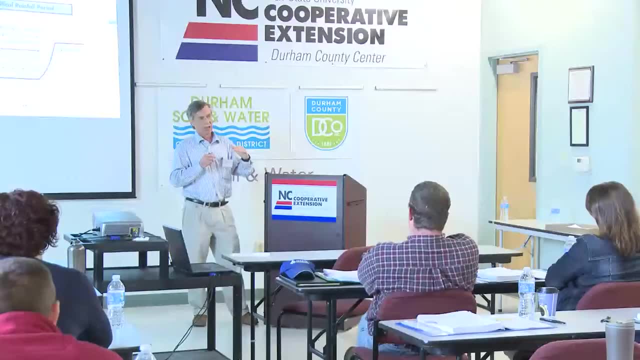 We took a drain mod there or we calibrated a drain mod model there and simulated then 40 years of daily water table data. So we had 40 years of water table data which we could interpret. We applied this technique to each year and said, all right. 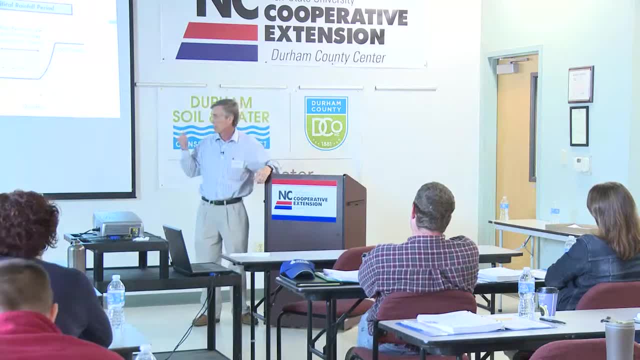 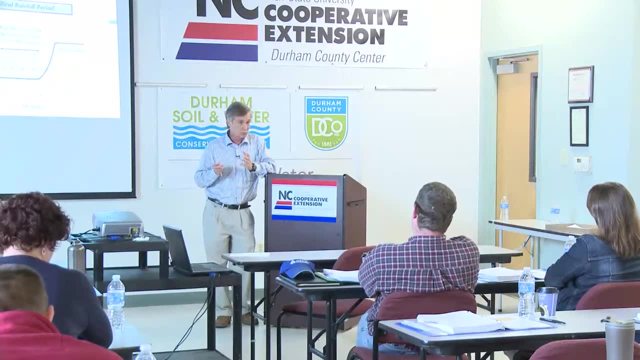 if we just did it for that one year, would it meet hydrology or not? at this site that meets at 95% of the time. We found with this technique it met using just one year. the conclusion you draw from that: one year. 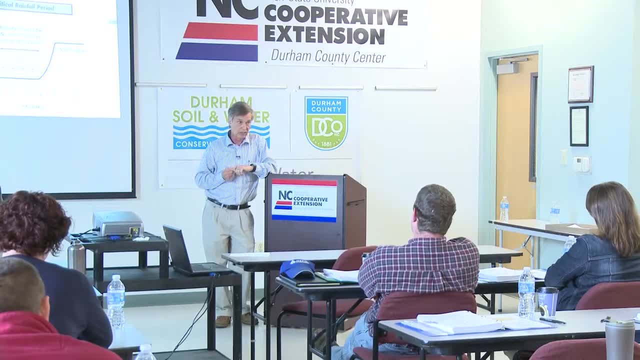 was correct in 85% of the years, Not the full 95%. The reason is that you have to exclude wet years with this, So you never get 100%. All I can say is: so we use it because it worked, based on that study. Okay, I just want a shorter recovery time for drought or either rainfall, that you don't really have three months. there's a shorter period that it's so important. Well, I can't argue that there's a shorter recovery time for drought or either rainfall. 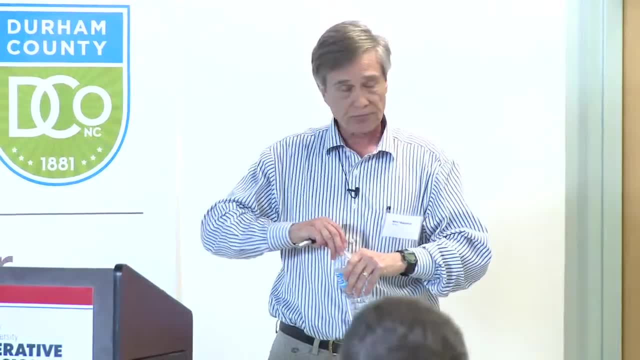 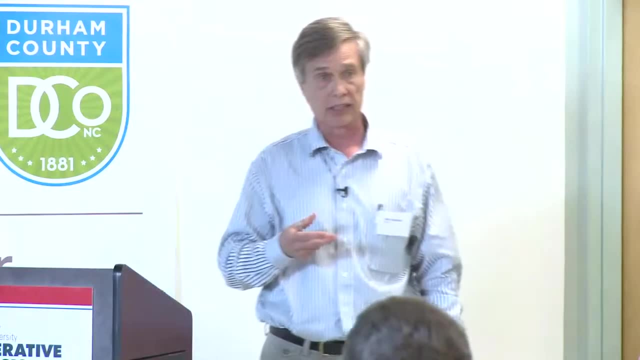 that you don't really have three months. there's a shorter period that it's so important. All I can say is this is what was recommended by that study and it looked like it worked in our case. I've talked it over with a man. 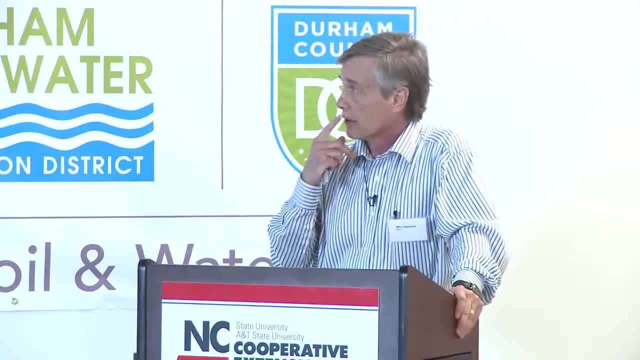 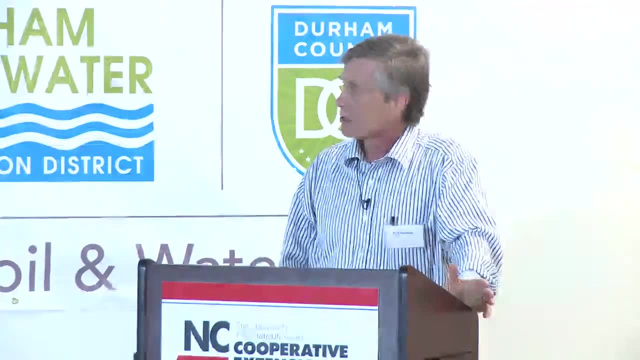 Paul Rodrigue, a USDA hydrologist, and he also recommended the three months. I can't. I have to go back to the Sumner study to see if we looked at the one month period. If we did, it did not show as good a result. 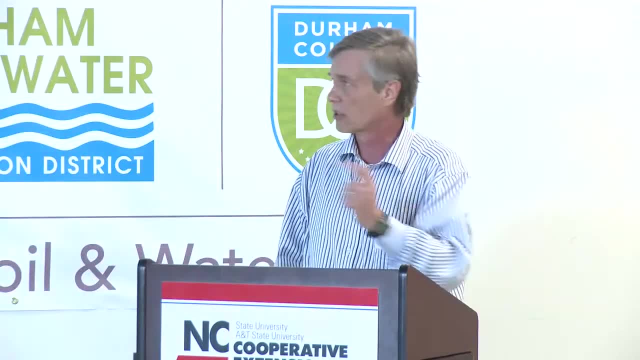 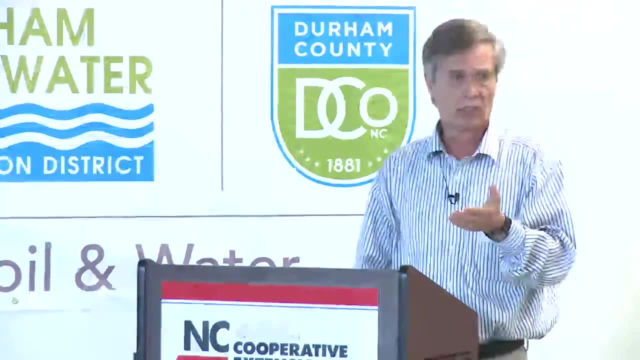 as this, And I don't really see that this is a difficult problem going back three additional months for rainfall. So what I can say is that if we look at three additional months for rainfall, at least it shouldn't be- And the rainfall. 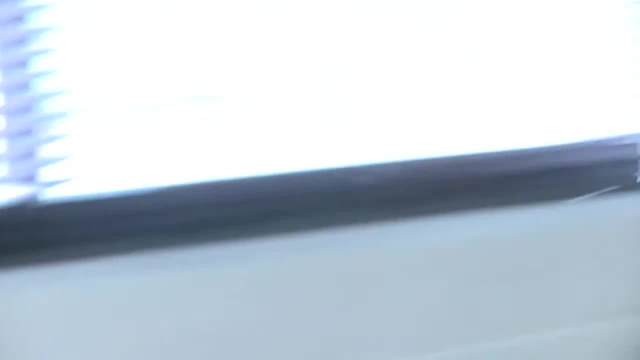 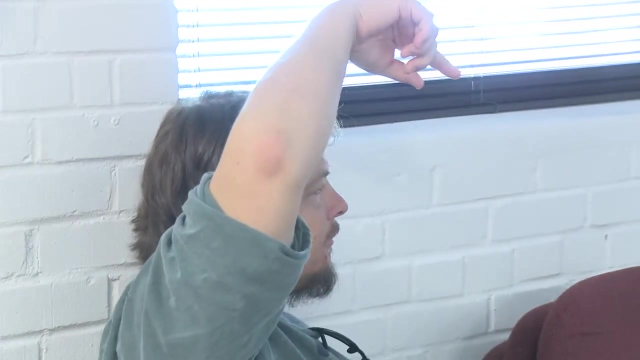 could be outside the growing season. Yeah, It looks like in the chart that you've included the month where the rainfall occurred. How come you don't use months one, two and three rather than two, three and four? That's from the graph. 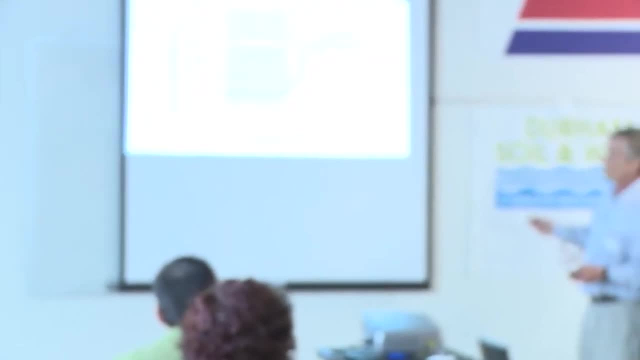 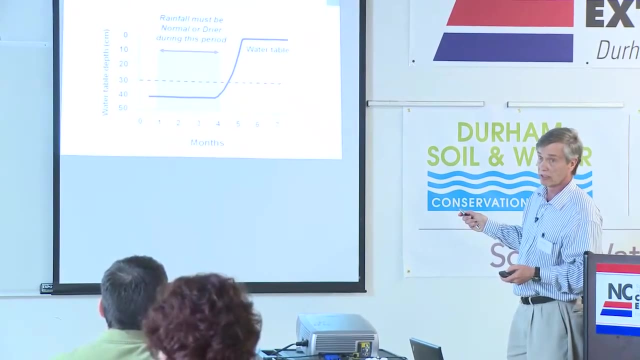 Okay, So it looks like the rainfall occurred in month four. The water table rose in month four. I bet The water table rose in this month. This is water table, not rainfall, now, And so you look at the prior three months. 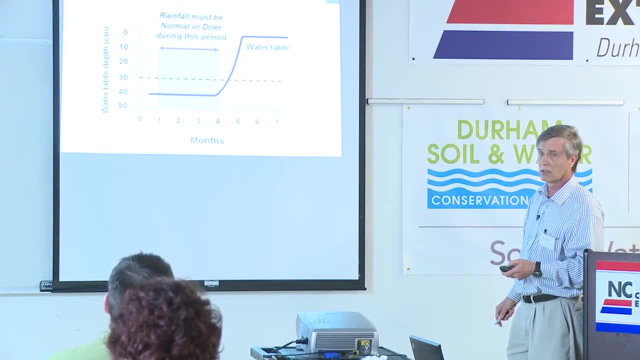 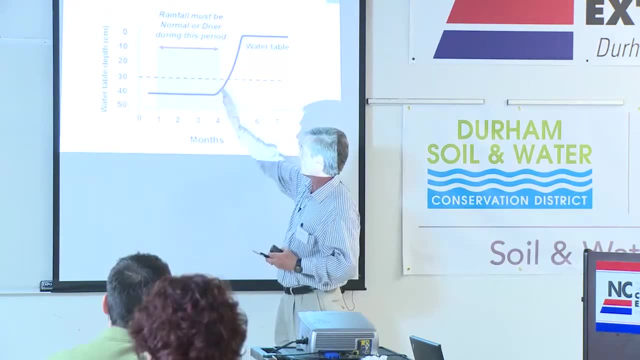 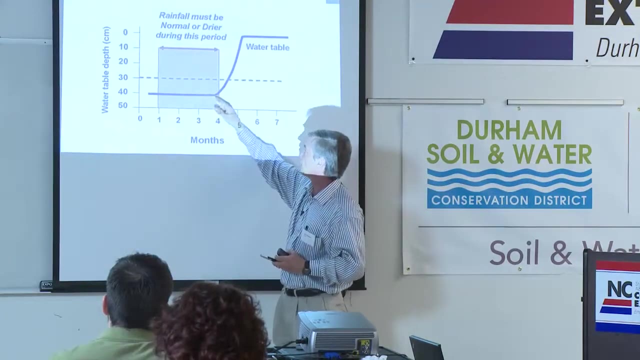 Right, And you said that you calculated based on when the rainfall event occurred that caused the water table to rise. Right? The water table rose in this month, So we look at the rainfall coming prior to the time that the water table rose. 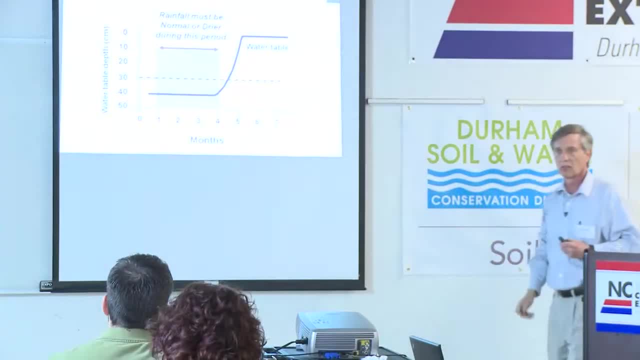 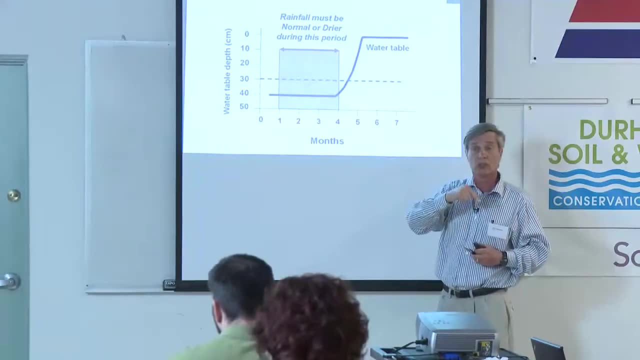 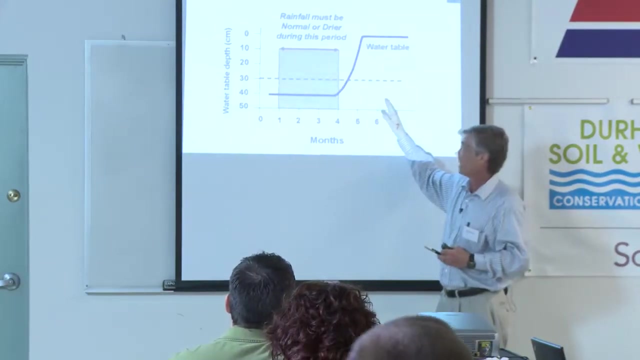 So the rainfall that basically created this rise- This not in the example I just gave you. You could- There is a procedure for doing that- Okay, So you could also include rainfall here. It didn't improve our predictability appreciably. 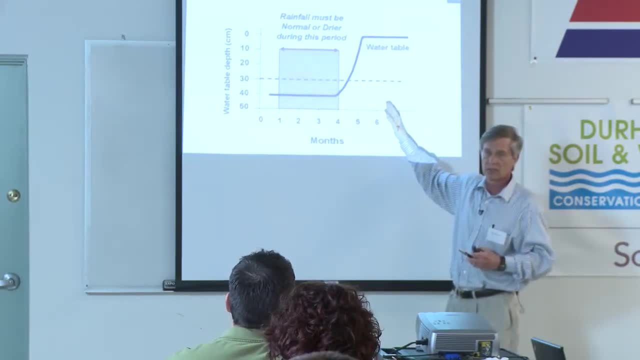 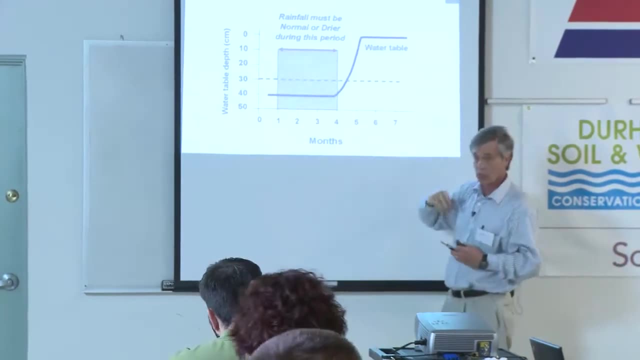 All right. One other thing. So there's different ways of doing this and they're preferred. I mean, all are appropriate. Yeah, Aren't there in this situation? aren't there trying to get around the? you know? 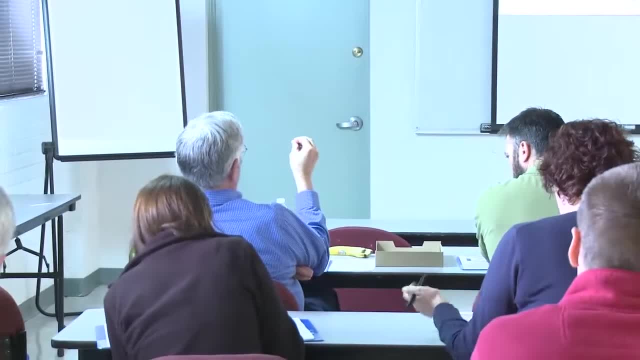 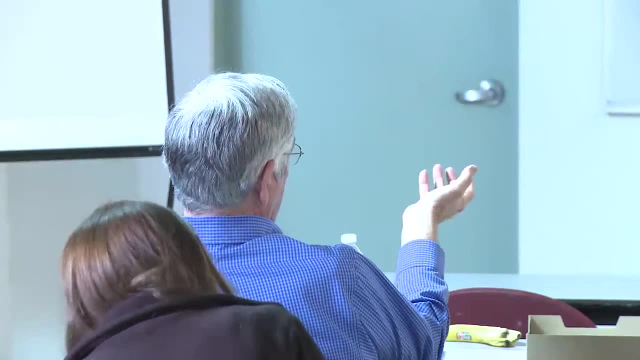 the trying to get around the problem of where people argue one way or the other that this, that our sites are being a necrology, plus the point we had earlier in that problem here: Lots of rainfalls, You run out there and you get. 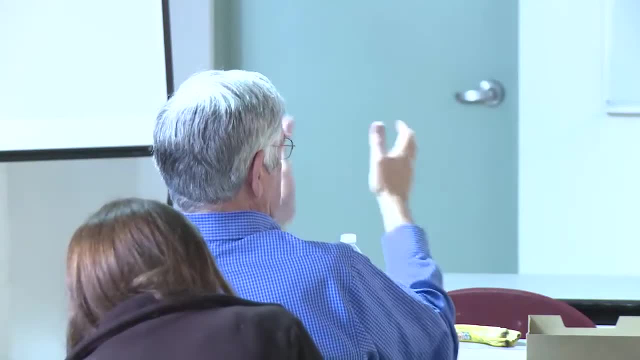 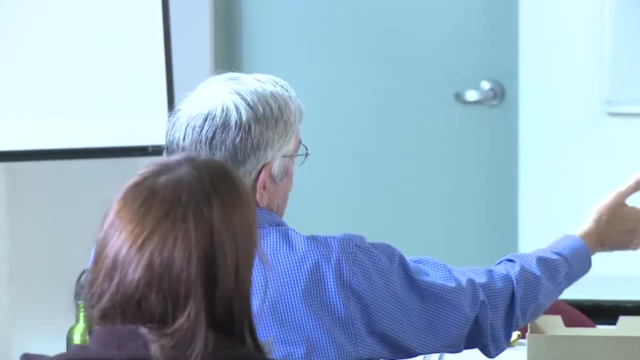 something bad. But in fact they're saying, over the long haul the system itself may fail, because this was just an anomaly. This gives you a way to really look and see, because organisms can't survive in one storm. So let's say you had this. 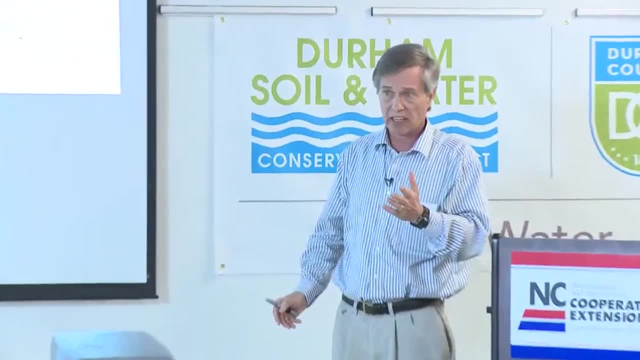 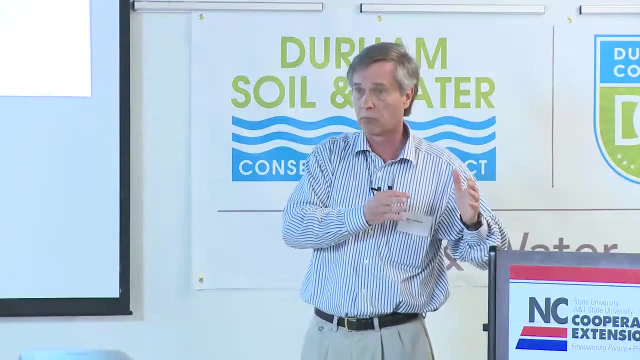 abnormal period that created a high water table. That's basically one event. There may be suitable events that you could use later in the year or earlier in the year that would be appropriate. So this is basically event-driven or event-focused. We're not focusing. on a year per se? Okay Yeah, Does it cause a problem if, like you, have a three-inch rainfall until it rises? but, like you have to base it off of, like what happened in, just because these values. 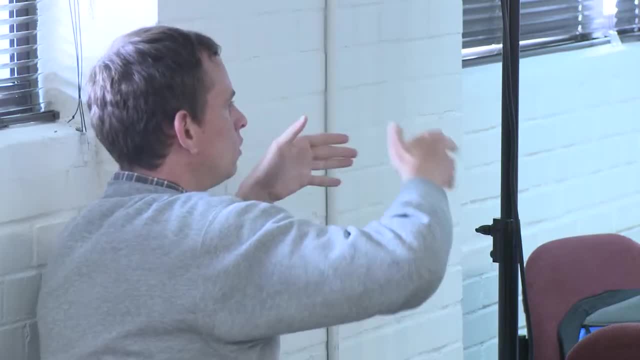 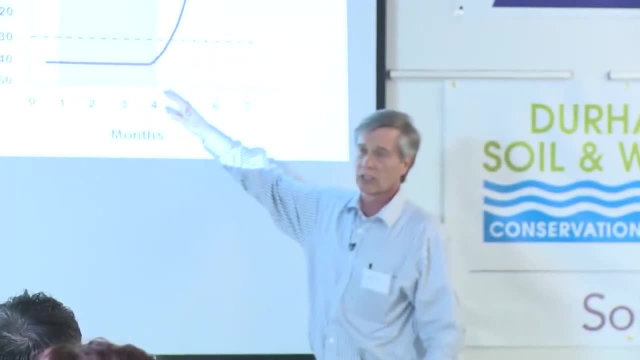 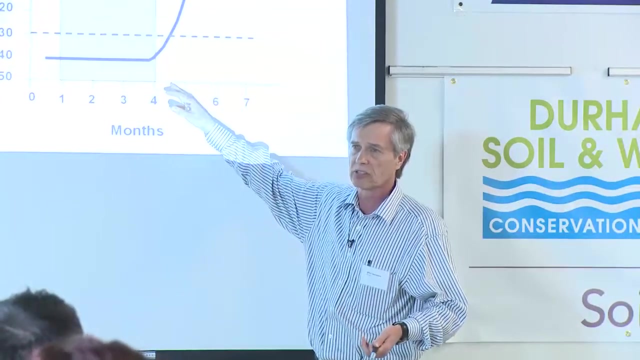 are based on just March and all those things. I don't think so. One of the techniques that we did look at is using partial portion of the month, And we found that that wasn't. that didn't appreciate. increase the accuracy of your predictions very much. 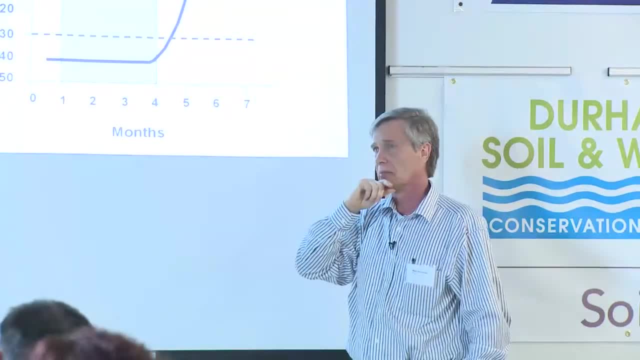 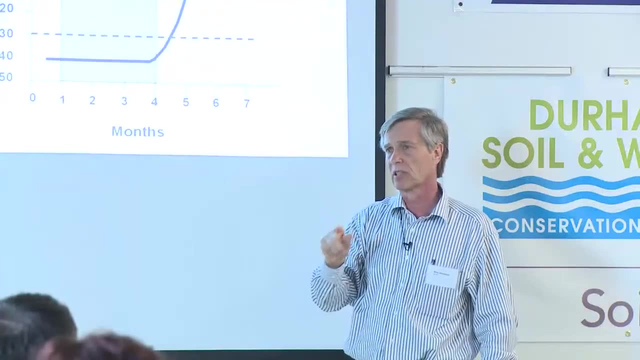 at all. Now let's see if it was an extreme event, But I don't. All I can say is: we considered that, but I don't think it's going to be a problem. You could look at this or include it. 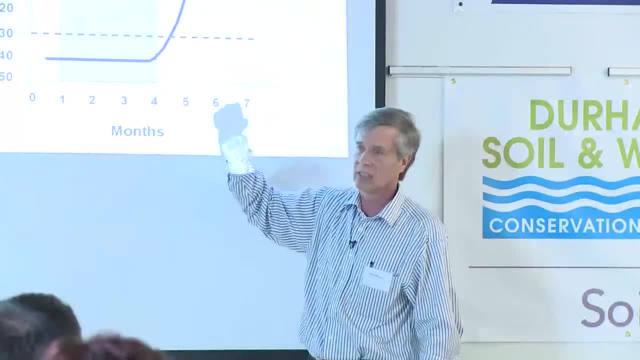 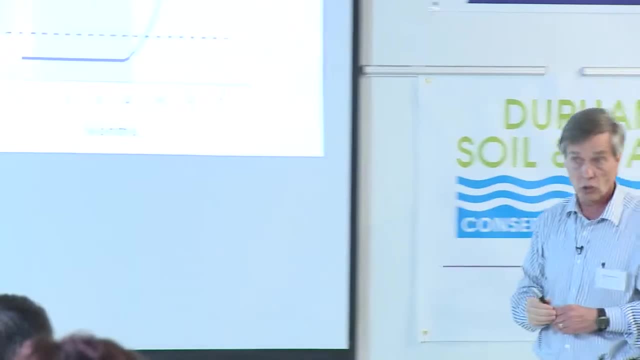 In fact, I think the student said: if anything comes within the first 15 days, eliminate it. Now, if it's after 15 days, you might want to include it, But that's a slightly different procedure than what I'm talking about here. 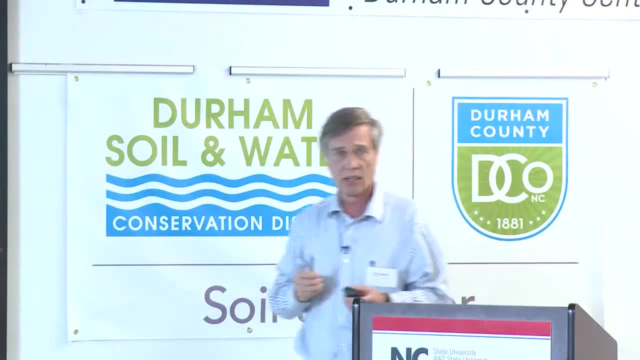 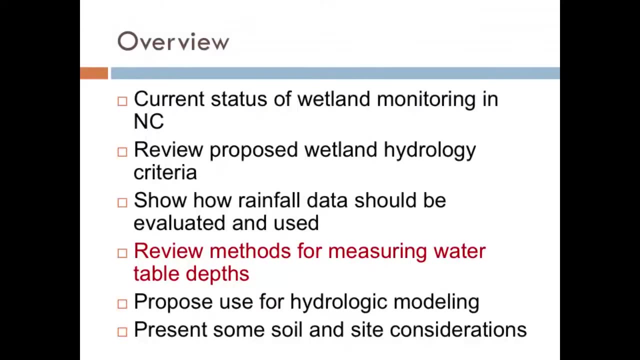 But it could be used if you wanted to Anything else. All right, See, rainfall is interesting. Remember that. All right, Now let's talk about measuring water table depths. I think all of us probably know how to do that. 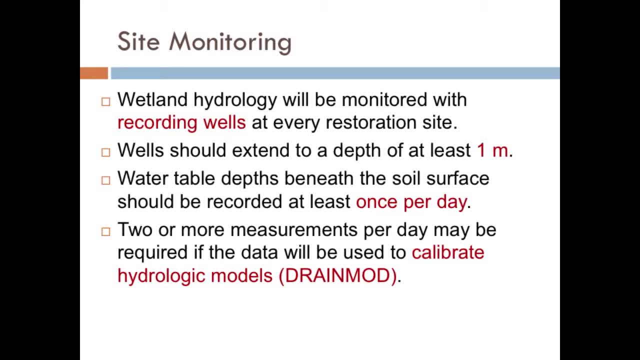 but let's just make a few comments here. Wetland hydrology will be monitored with recording wells. That's what we're recommending. They're readily available. The wells should extend down to a depth of one meter, If it goes deeper, obviously. 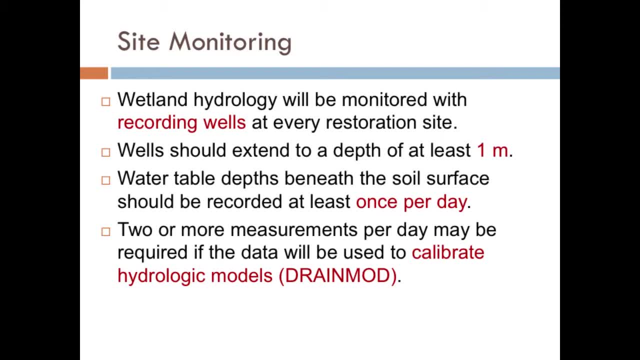 you're going to have to measure them once per day. If you're doing modeling, you might want to read them or have them set to read more often than once a day, twice a day to up to four times a day, That is. 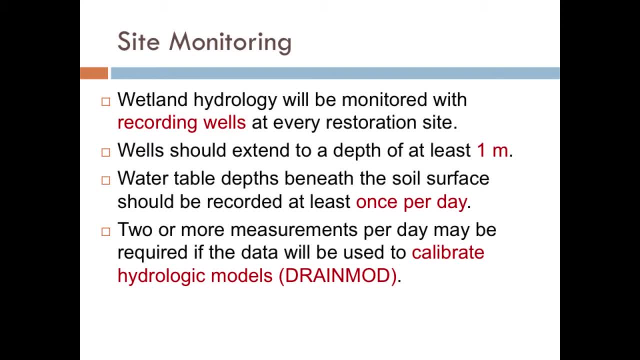 if you're using the data for drain mod, I should say all of our wells that I've used in research. read once per day. You can still do drain mod simulations, but sometimes more frequent measurements might be warranted. How many wells do you install? 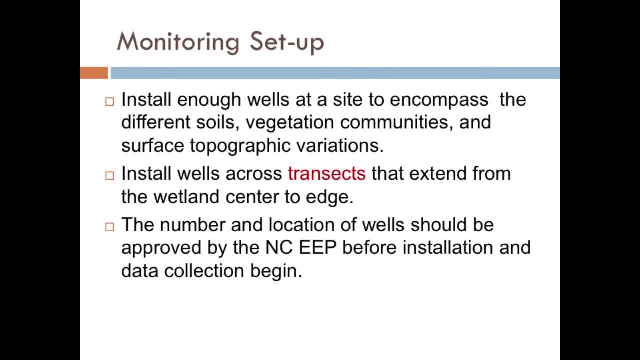 We don't have a set number, but we want you to install enough to encompass different soils, vegetation communities and surface topographic variations. In other words, you don't necessarily focus only on the depressions where you expect it to be wet. 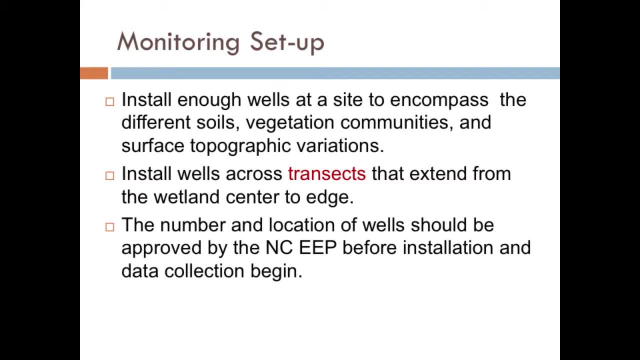 If you want some guidance, we recommend installing wells in a transect And the number your sampling plan giving number and location of wells should be approved by the EEP or at least run by them, before you actually go into the expense. 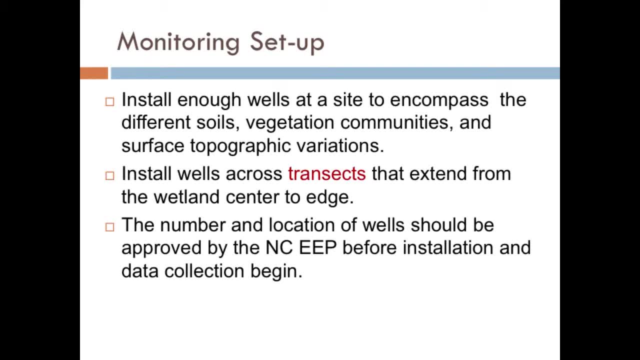 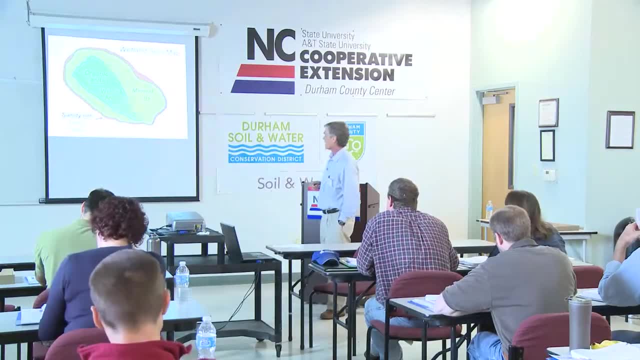 of putting the wells in a transect. As far as I'm concerned, talk to the regulators first to make sure that they will agree to accept the data. Let's give you an example. Let me give you an example. Okay, this is: 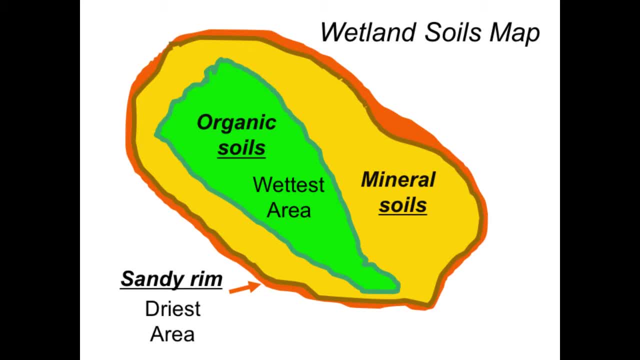 a Carolina bay with obviously organic soils in the middle. This would be the wettest part of the wetland mineral soils here, and then a sandy rim which is just a little rise on the outside. So this would be the dry area. 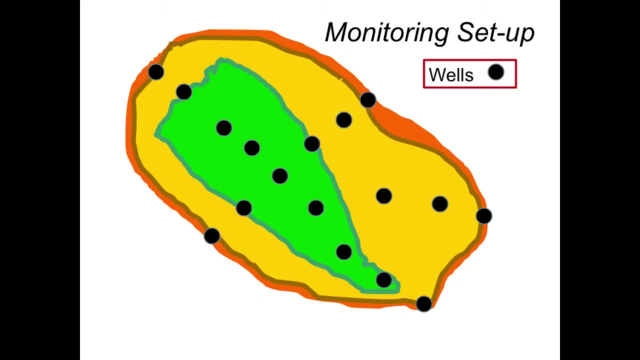 wettest area here. If you wanted to instrument the site, you could put, I think it's, 17 wells. This would be two transects, one along the long axis. This would be about a mile and a half long in this case. 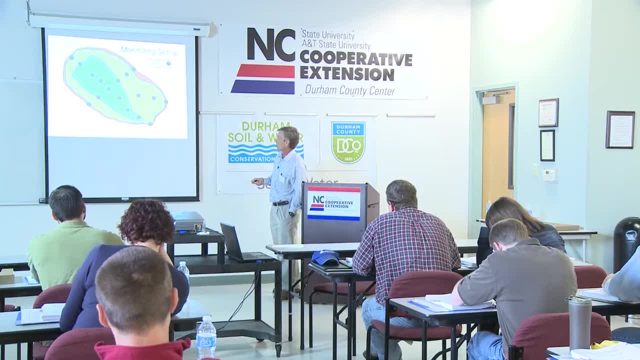 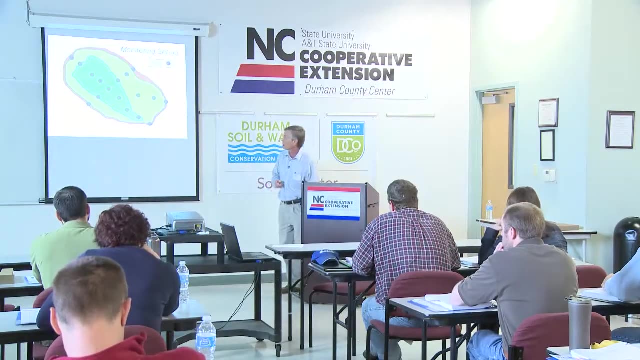 a mile wide, So it's really not overly intense well placement. This area was left alone so we threw in a few more wells here, But this again would be a well design where you're using transects and hitting a gradient of wetness. 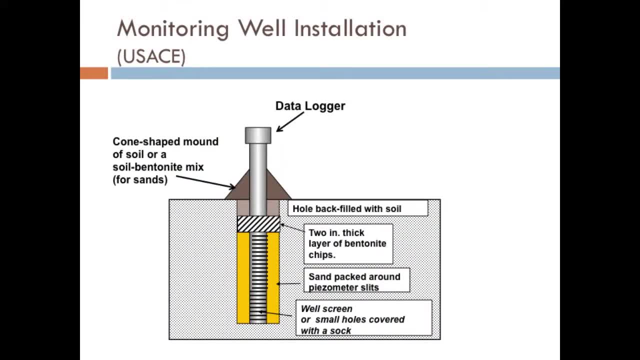 going from the middle to the edge. Unlimited budgets. you can add many more Wells, I think should be installed following the Corps of Engineers guidelines which are shown here. I don't know if you're all familiar with this or not. 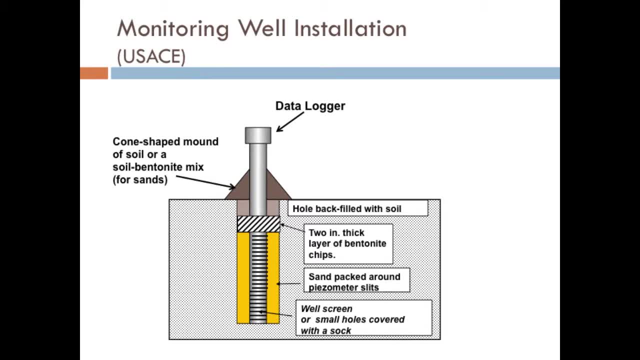 but we'll put in a well to a depth of one meter by augering a three-inch diameter hole. We backfill the slotted portion of the well with sand, cap it with a two-inch layer of bentonite, which is swelling clay. 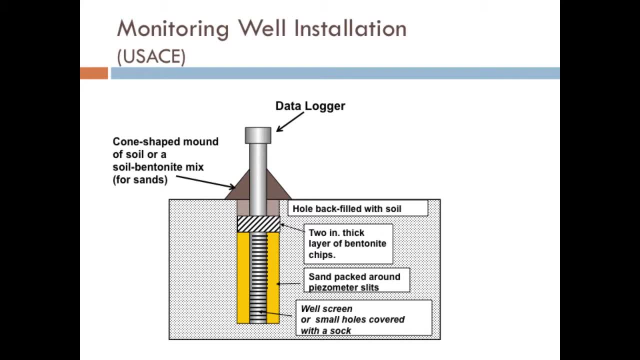 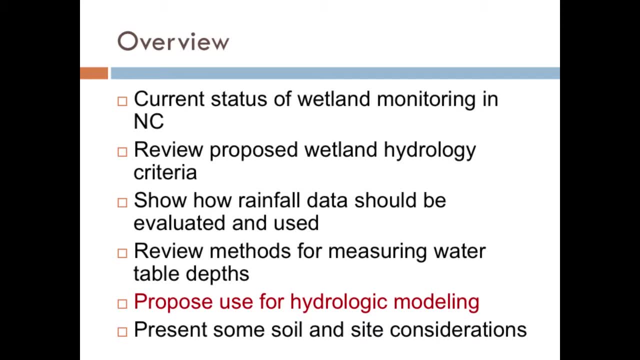 and the surface water should not be coming down and we're basically good to go. Okay, we had on our group about half the group familiar with modeling, and so modeling was mentioned in our standard, mainly reflecting the ideas of Wayne Skaggs. 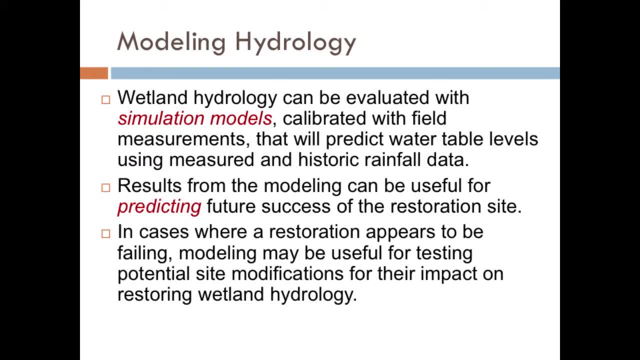 He believes that wetland hydrology can be evaluated with simulation models such as DrainMod, which calculates water taking from water table levels, As long as they're calibrated for the sites, using on-site measurements and then plugging into the model your historic 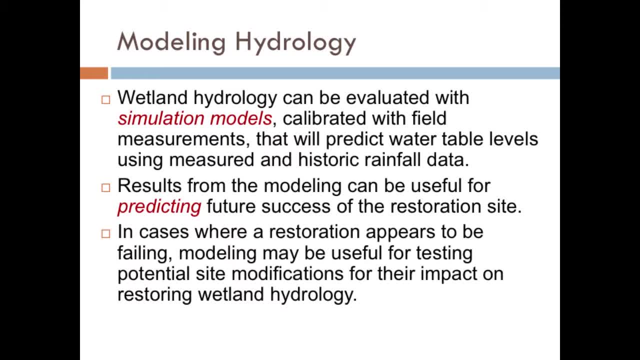 rainfall data to get 40 years or so of water table data. Once you look at that record for a restored site, you should be able to see if you're likely to meet wetland hydrology or not. I think that's a good example. 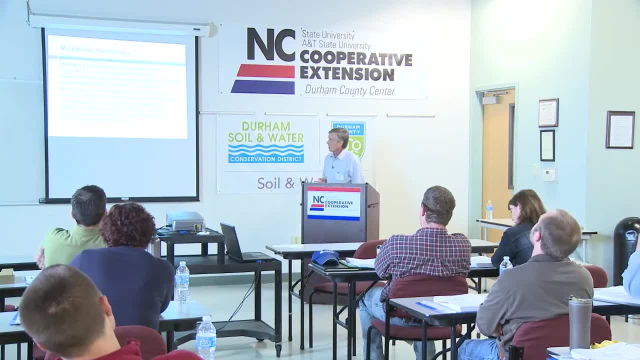 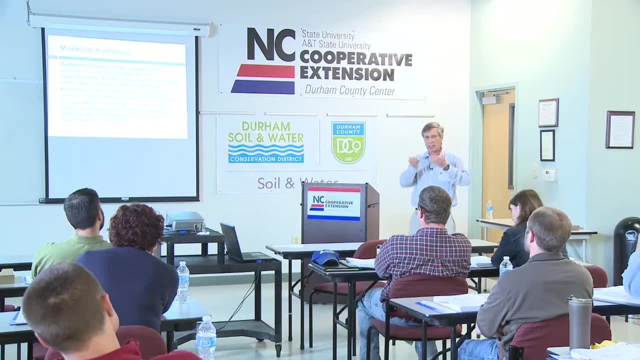 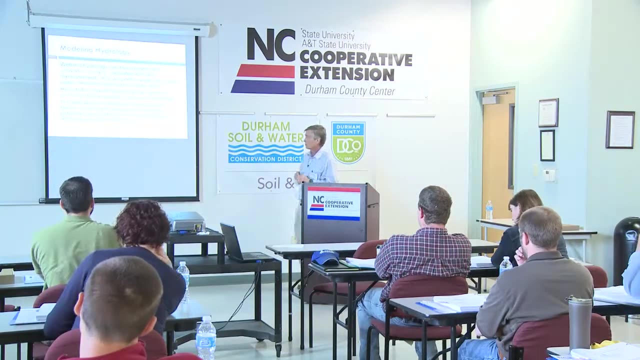 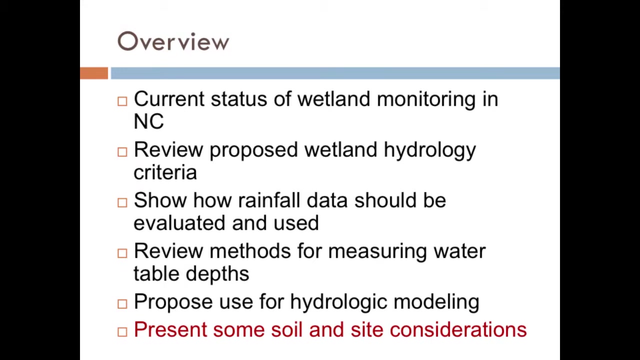 of a restoration site. Also, if you're finding that you're coming up a little bit dry, you could adjust things in the model like surface roughness or surface storage and see if these site modifications might raise that water table a little bit more for you. 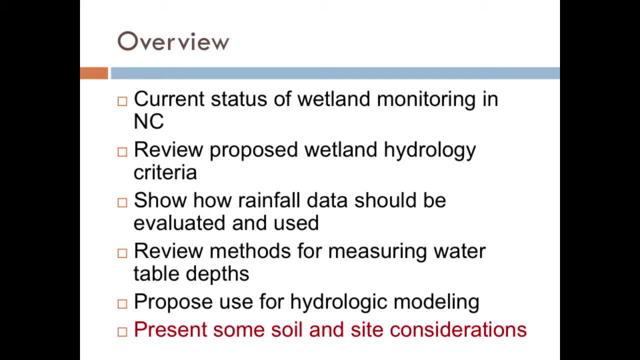 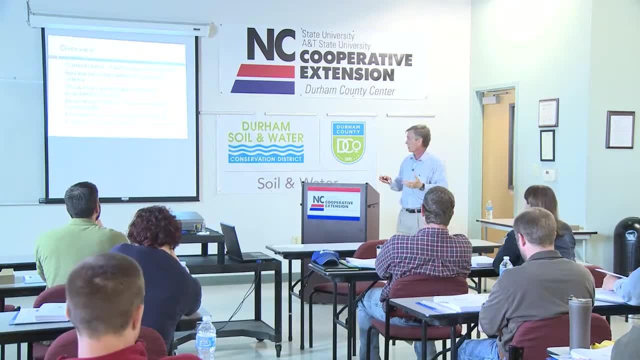 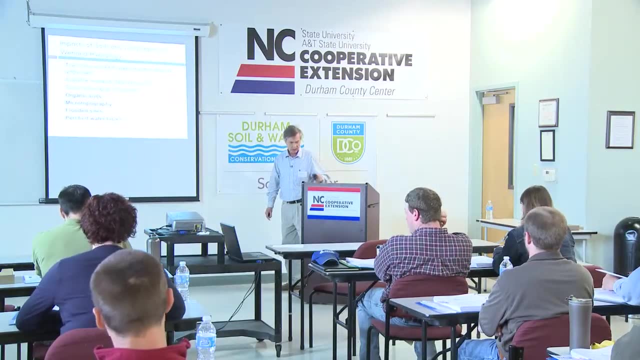 Got it. The other thing that the EEP asked us is to give them some guidance on soil and site considerations. Of course, we wanted to stick with stuff that we felt comfortable with and unfortunately it didn't cover all the cases they wanted us to address. 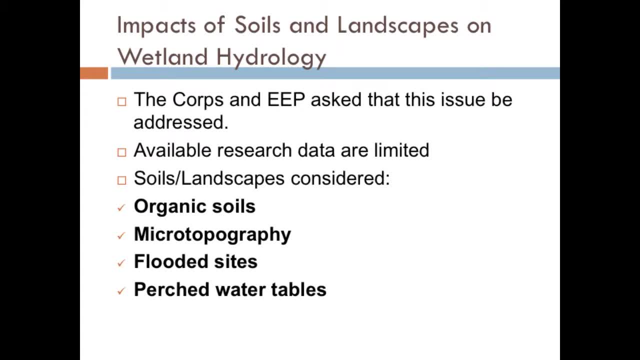 but let me just run by some of these for you. So they wanted us to address these issues. They wanted us to address organic soils using microtopography. comments on flooded sites. I won't have time to say anything about perched water. 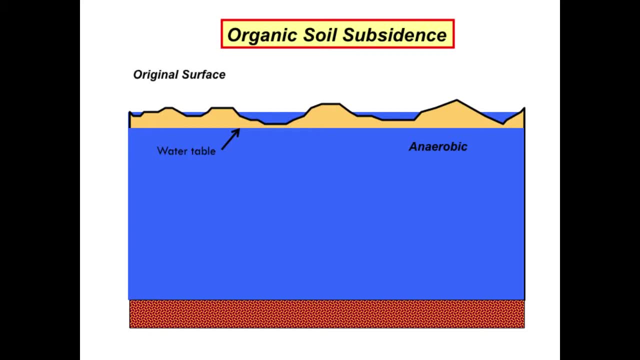 tables, but we did address it in our final product: Organic soils. We've got a lot of these in North Carolina and they're in North Carolina. We've got a lot of these in North Carolina and we have a lot of these. 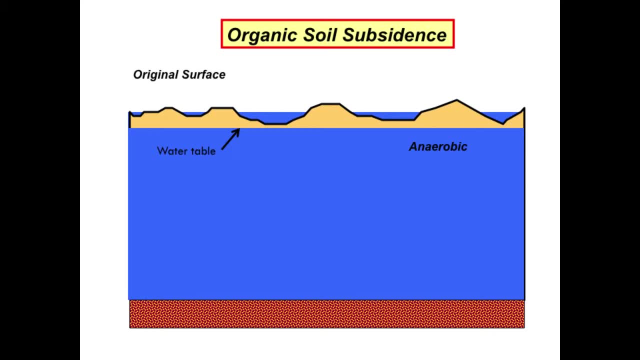 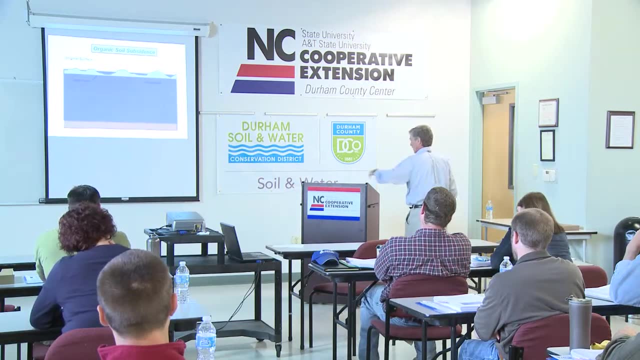 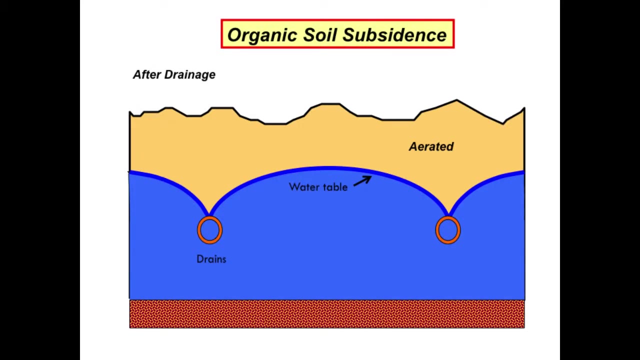 in North Carolina. So we have a lot of these in North Carolina. We have a lot of these in Northern Carolina, And we have a lot of these in North Carolina, and we have a lot of these in Southern Carolina. We have a lot. 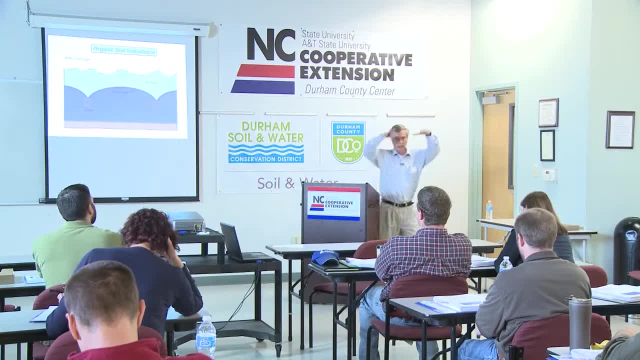 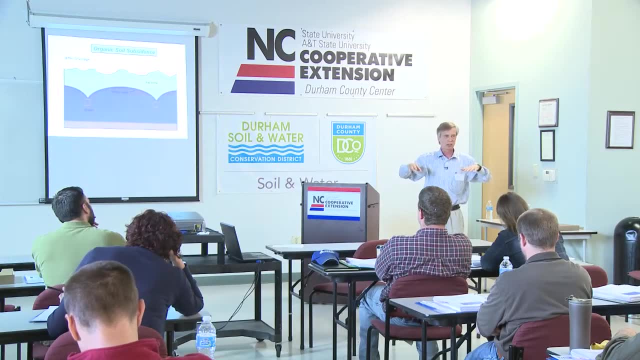 of these in North Carolina, So we have a lot of these in North. when you lower the surface, It's like you're doing a back float in a swimming pool and the water goes down, You hit the bottom and the same thing happens here. So the point is, when you drain organic soils, 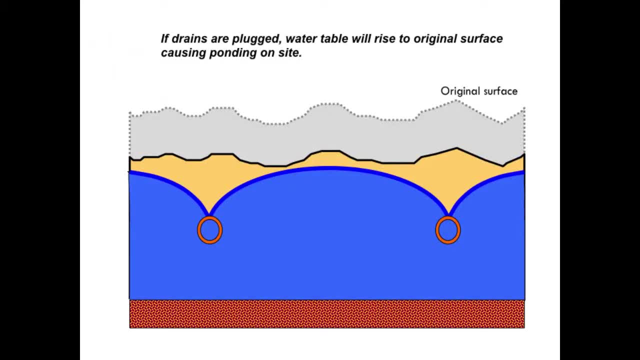 the surface goes down, All right, and it goes down a little bit more each and every year. Now, if you come in and restore this site by plugging the drains, where is that water table level going to rise? to The current surface, which is here, or the original, which is here? Huh, Yeah, it's a quiz. 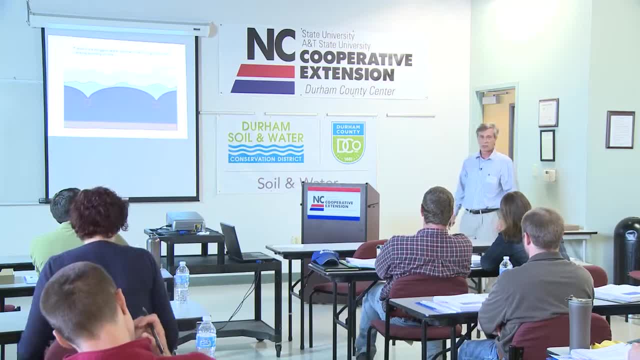 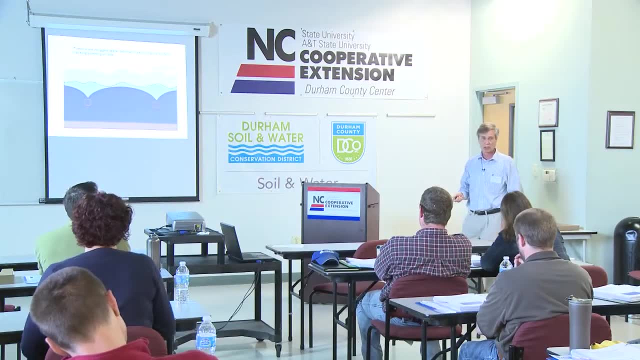 question. It could go back to the original, assuming there's not massive drainage in the surrounding area. That's correct. This might be three, four or five feet above the original surface. Okay, so you have to allow for the fact that if you just plug the drains on organic soils, 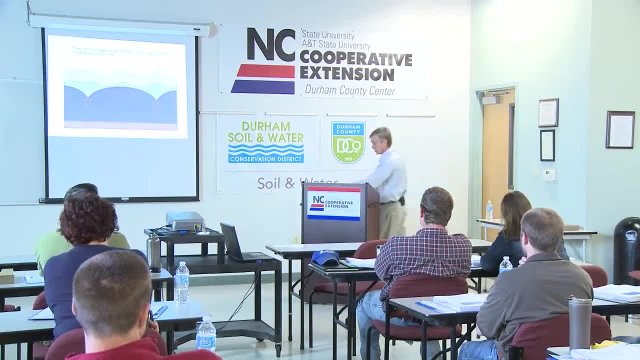 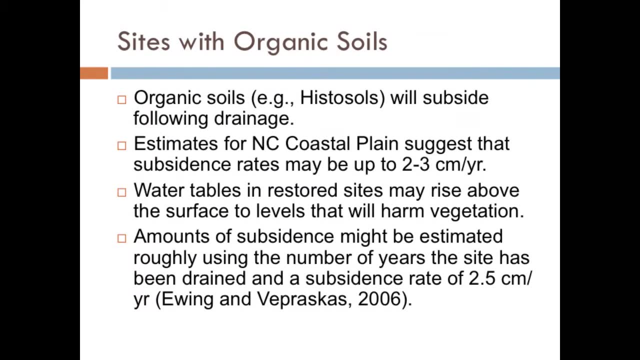 The water table could rise above the surface and you'll create a lake. Now the organic soils or the histosols subside, The process of surface lowering, is subsidence, at least in the soils community, Subsidence, I think, in the ecological community. 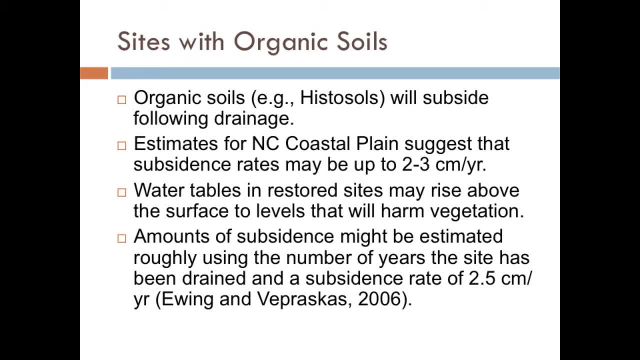 Our rates. we estimated some rates of subsidence in our organic soils and came up with about 2 to 3 centimeters per year, That's about 1 inch per year. Water tables and restored sites again may rise above the surface. 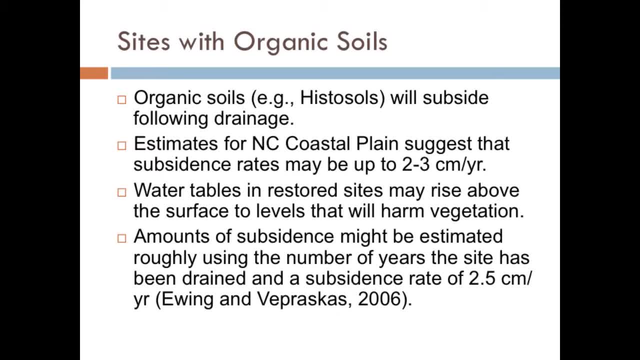 to levels that harm your vegetation. It might kill your trees if you create a lake. So you might want to estimate the amount of subsidence that has occurred at a site And to do that, what we're suggesting as a rule of thumb. 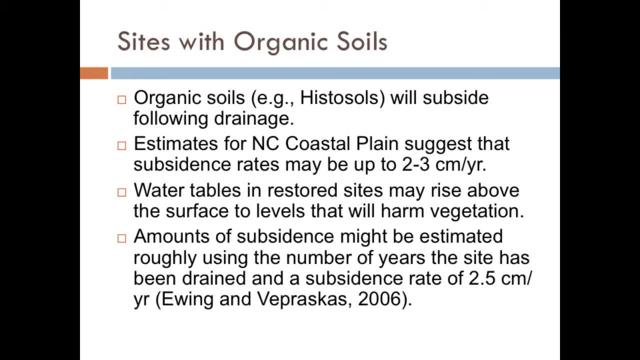 and it's been published. take the number of years that the site's been drained and assume that you get 1 inch of drop each year. So if a site's been drained, if it's not been drained for 30 years, as many of ours have, 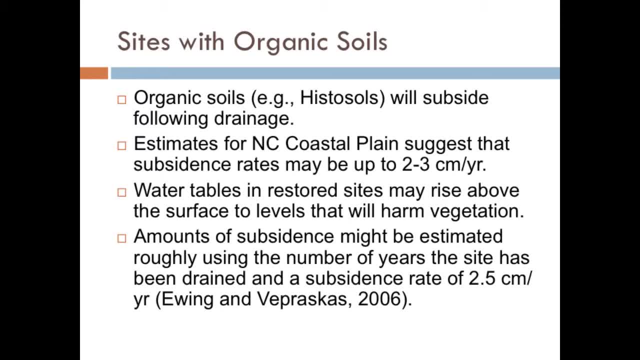 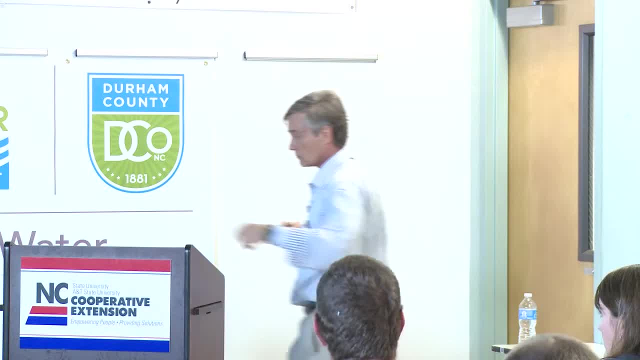 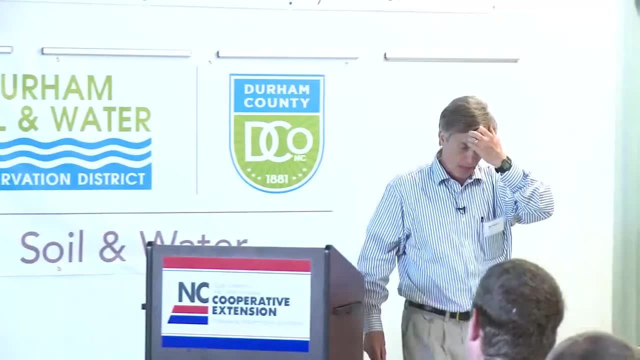 the surface has been lowered by about 30 inches. Okay, A rule of thumb. So if you restore that hydrology, the water table will rise 30 inches above the surface. So we felt pretty safe making that recommendation. Somebody called me one time and says: why are our organic soils easier to restore to wetlands than mineral soils? And I said, heck, yeah. They said why? Well, because you've got a lot of water, You've lowered the surface quite a bit, so the hydrology's almost a no-miss situation in restoring. 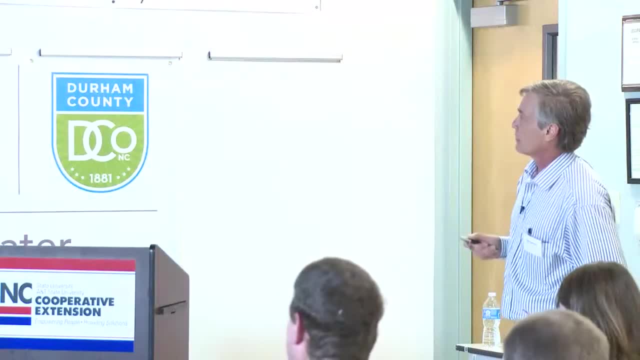 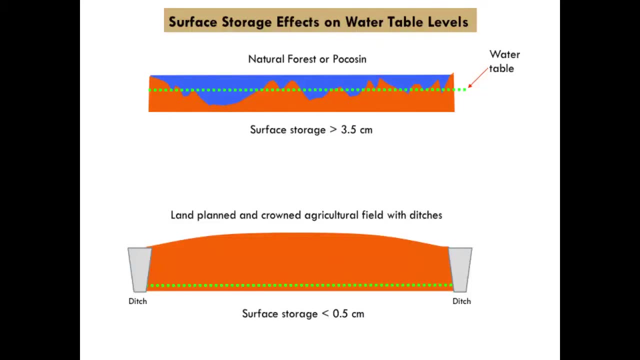 Okay, whoop, running out of time. Surface storage effects. The engineers are very big on surface storage. Now let's just explain this. If you go into a natural wetland, it's very hummocky. Trees tip over, they make depressions and those store water. 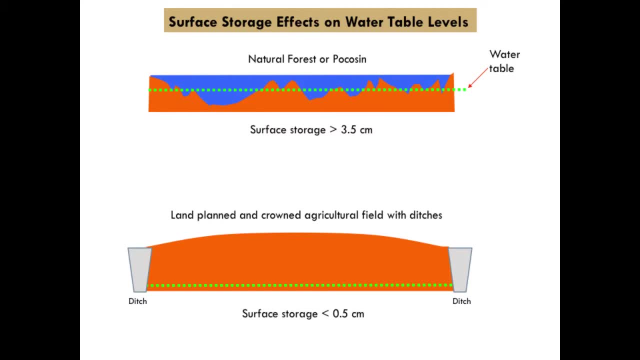 And, as a result, they will force water into the ground. You get the high water tables on these natural hummocky wetlands. Now, when a farmer goes in to drain the site, he or she will put in drainage ditches and crown the field. 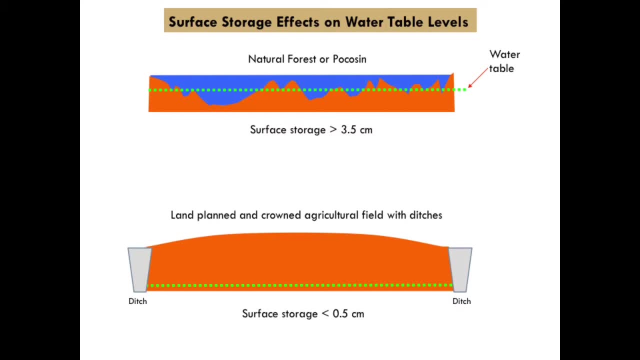 make it a base, a football field, virtually removing all surface storage, And this contributes to deeper water tables. So when you restore the site, particularly if you think it's going to be a little on the dry side, the engineers recommend that you add or recreate some of this surface storage. 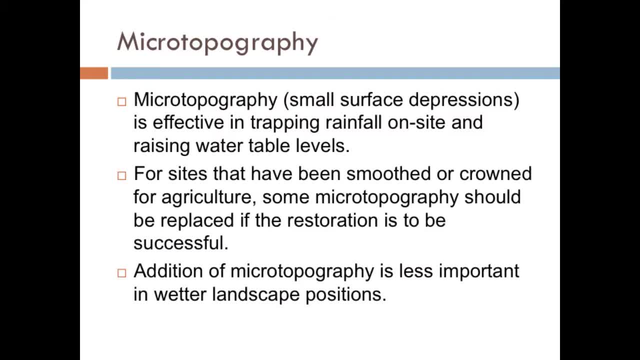 Attrap your water, raise your water table. This is what a restored surface storage site looks like. Okay. Okay, You can see it has to be done with earth-moving equipment, or plows in this case. So they took a plow, made some curlicues, took a bulldozer and made little ponds of depressions. 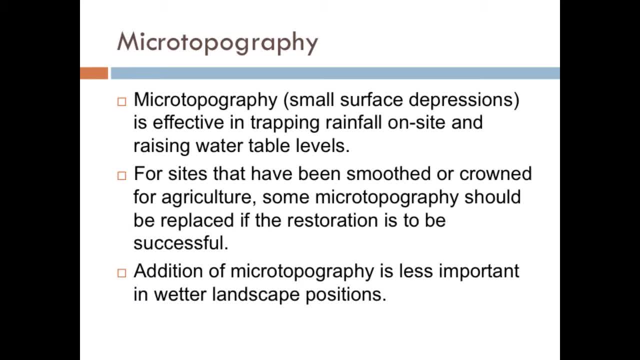 They all seem to be effective in trapping the water and forcing it into the ground. So, surface storage, Mite topography or surface storage, these small depressions 6 to 12 inches deep, over an area of- oh, I don't know- 3 to 6 feet or more, are effective. 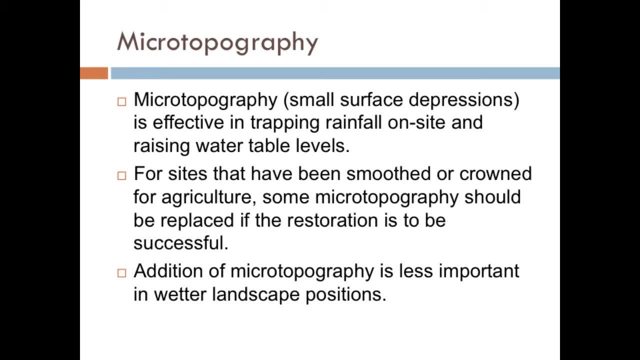 They're effective in trapping rainfall on site and raising the water tables. In fact, sometimes they'll go up about 8 inches if you add storage or take it away. So for sites that have been smoothed or crowned, I think you should replace some of this surface storage, if you can afford it. 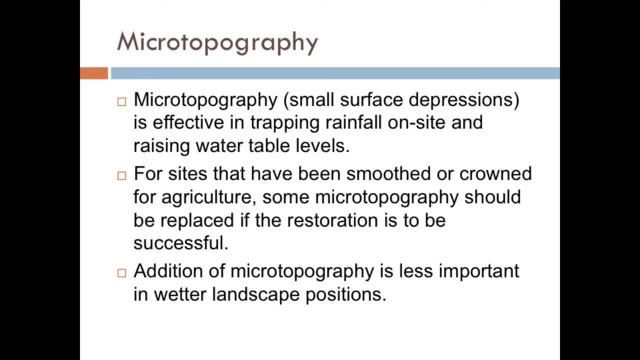 Now, if you are in a very wet location and are sure it's wet, then the microtopography or surface storage is probably less important. So I don't think it's critical in all cases. At least, that's what some of our studies have shown. 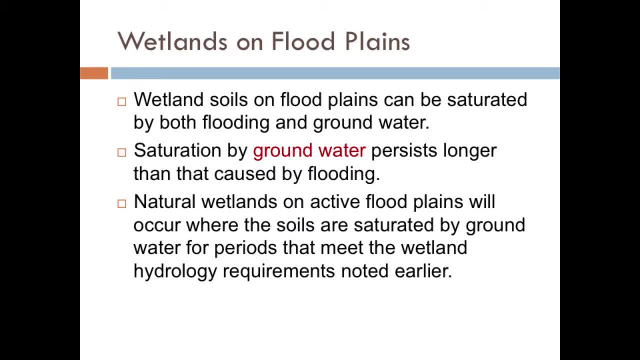 Now wetlands on floodplains. I'm a soil scientist, I look only at the soil, and so that reflects the following comments. Now you know that wetland soils on floodplains are saturated by both flooding and groundwater, And in my opinion, the groundwater is very important. 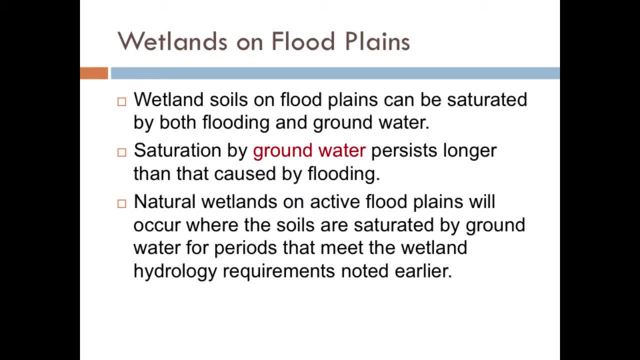 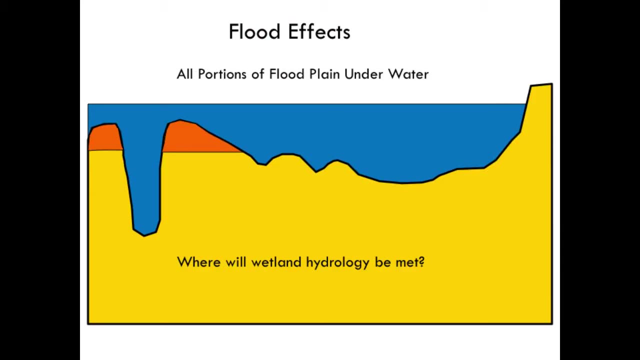 The groundwater causes saturation and persists longer periods of flooding in many cases, And the natural wetlands on floodplains are going to occur where the soils are saturated by groundwater for periods that meet or exceed the hydrology requirement. In other words, this is the floodplain of Tar River near Greenville. 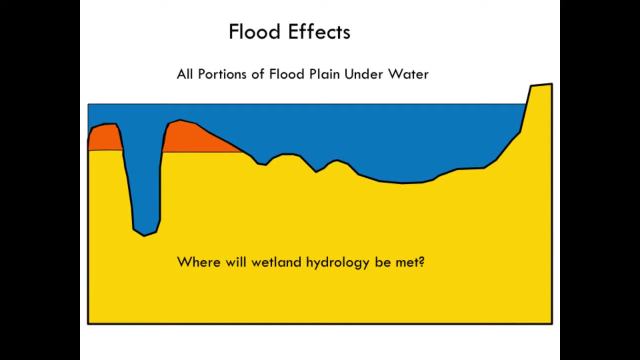 So we've got the channel, the levee. I call this the back plane and this would be my back swamp. So this would be a big flood. let's say, after Hurricane Floyd, All the area is inundated. but are all these areas wetlands or would they be jurisdictional? 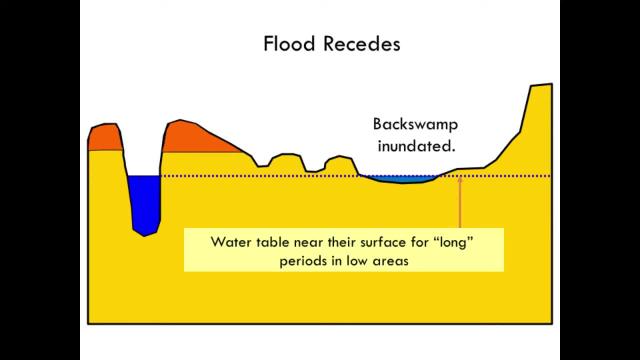 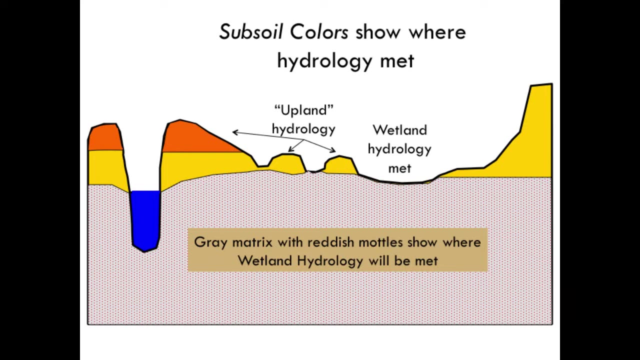 wetlands? The answer is no, As the water table, as the river subsides, the groundwater will have a level, something like this: The levee and the high spots on this back plane pop out pretty early If you look at the soil color patterns across this landscape, the gray colors that we associate. 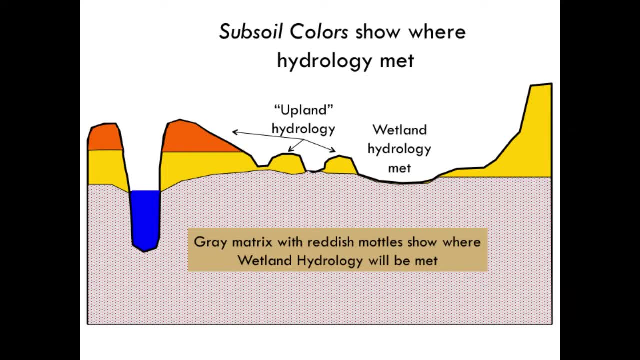 with wetland soils will follow a pattern that looks something like this: Okay, this is just obviously a cartoon, but I think it's based on field observations. You have gray colors in the back swamp, the area that stays ponded for long periods. 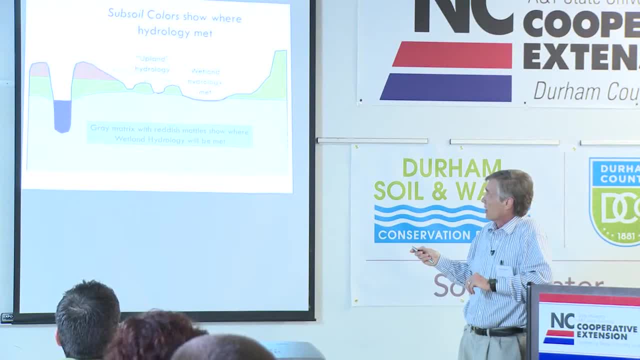 You'll meet wetland hydrology here, and you'll have hydric soils here as well. In the back plane, you'll only have hydric soils in the low spots, okay, and this may be where you meet wetland hydrology. 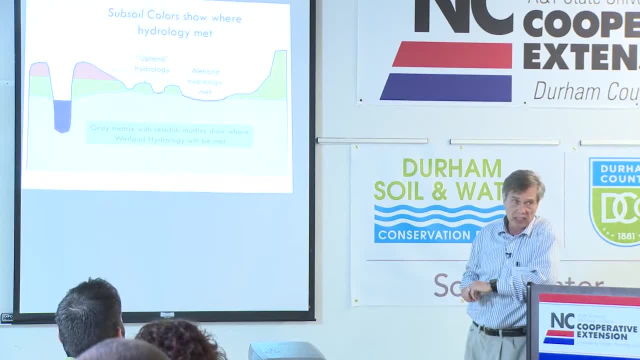 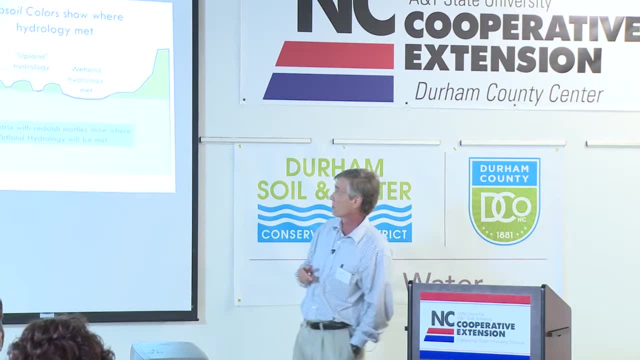 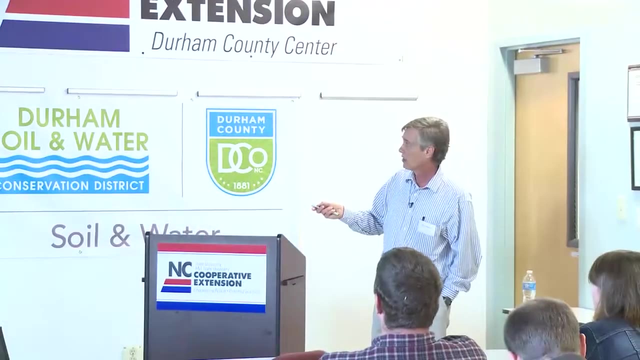 On the levee and on the high spots of the back plane, you probably will not meet our hydrology standard okay, unless you really keep the floodwaters from draining off. So the point is: don't expect that, Don't expect to meet this standard at all points on the flood plane and that's okay. 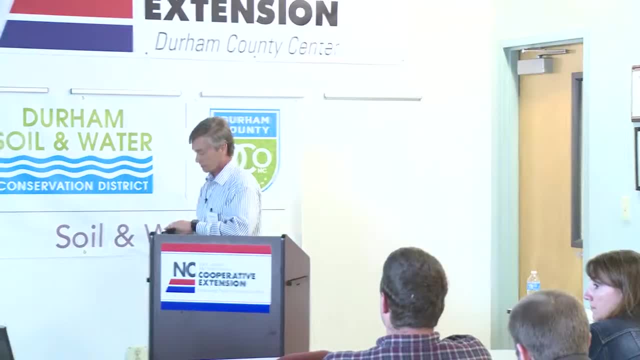 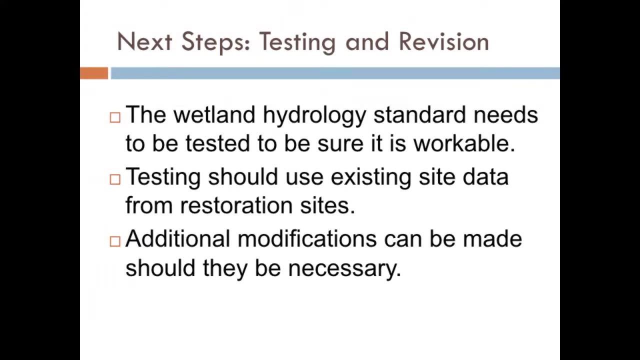 You aren't going to have hydric soils at all points on the flood plane either. Okay, the next steps. as I said, this is not an official policy at this time. I think I'd like to see it tested using some of the data in the EEP's database to make. 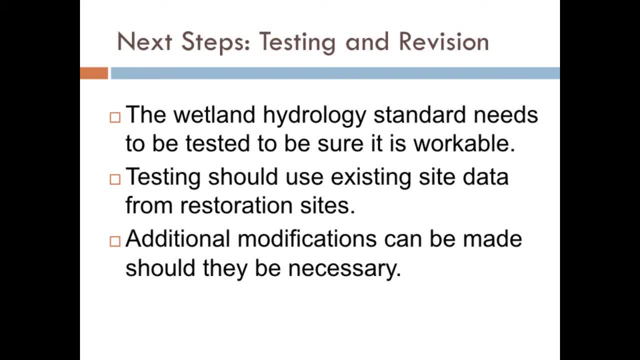 sure that it's a reasonable standard and that it's workable for the regulators to use. I think testing could be done on existing site data from the restoration sites. We put in a grant request to do it. I am very willing to make additional modifications if you have comments or things that you feel. 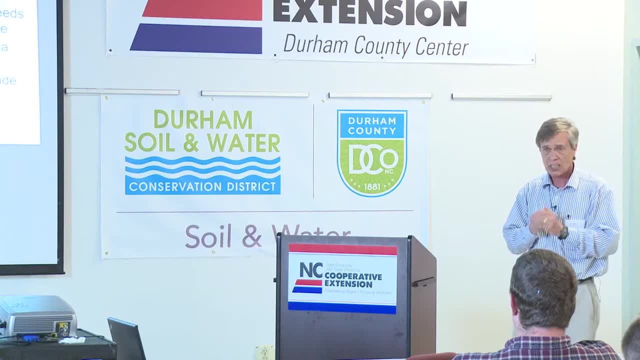 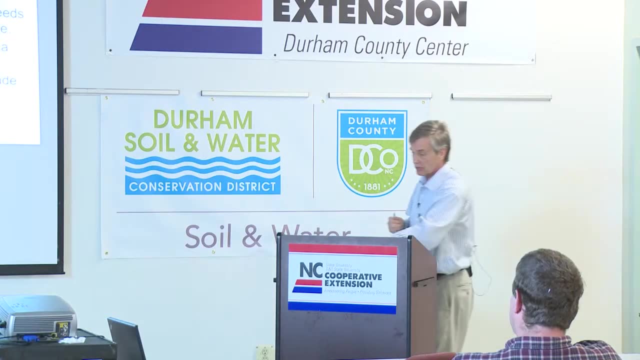 should be changed, let me know, and we'll certainly consider it Right now. I'm hoping to see somebody use this in the not too distant future. Okay, I think that's all I wanted to say. Thank you very much.